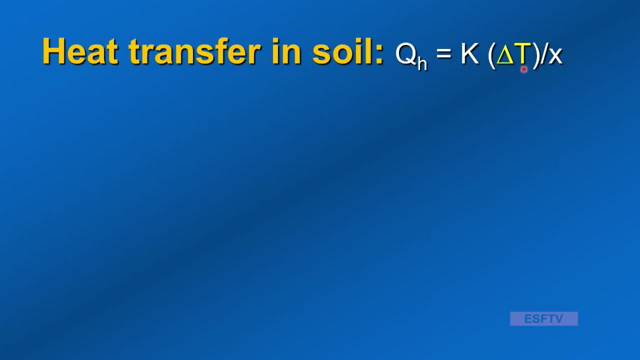 as proportional to K, delta T over X, and we'll kind of go through this. So what is this heat transfer? So we're looking at QH, the quantity of heat transferred across a unit cross-section, across an area right, And so per unit timing. So you know this. 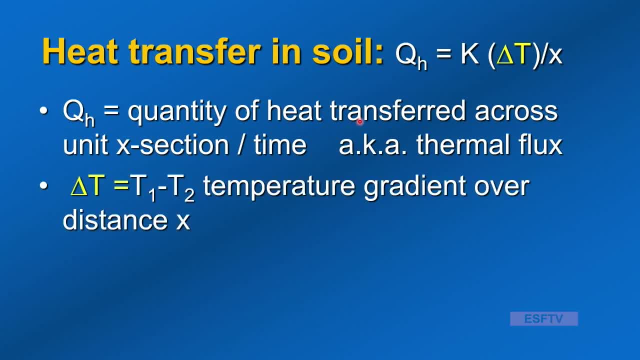 we'll know it soon, is something called thermal flux, And the other part of that is the change in temperature. You see part of that delta T, so the difference in temperature between one end of that space and the other, and this is a gradient. The greater that gradient, the greater the rate. 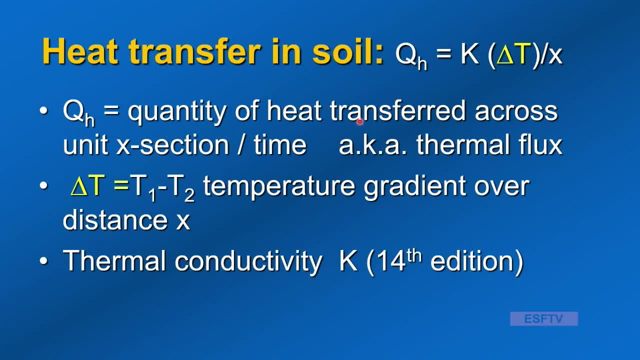 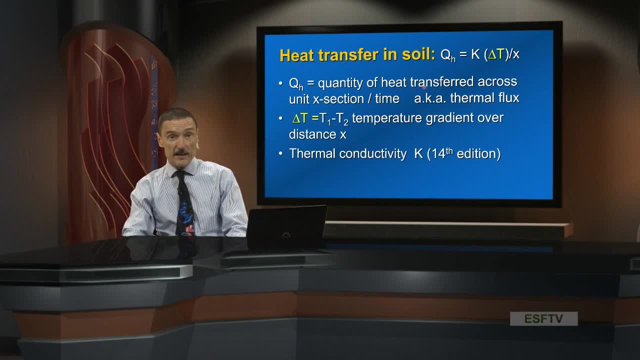 of transfer And conductivity, K. So this is in the last edition of Weil and Brady. we used K and this was this. So this is a way to express thermal conductivity. We've already looked at K, the expression of conductivity for saturated and unsaturated flow, and now we think about that in terms of flux of 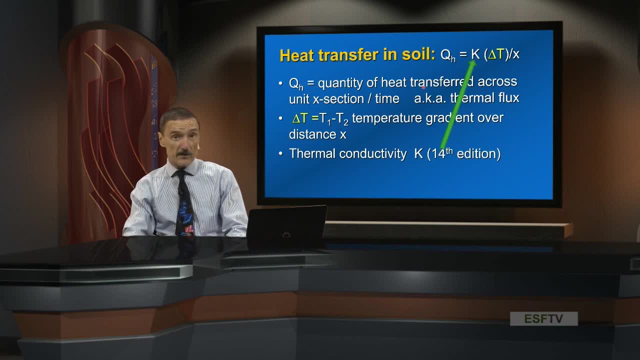 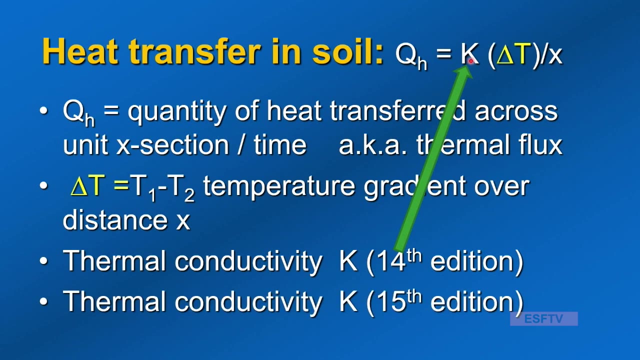 temperature and heat energy. And so there it is. There it is in our equation, right, We have K, and now here's where K is. So this is thermal conductivity, and this is expressed as a determining factor of heat transfer. So in the 15th edition this is lambda. So for some reason now it's lambda, before it was K. 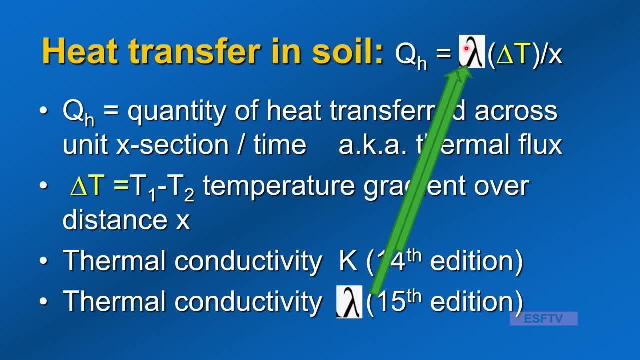 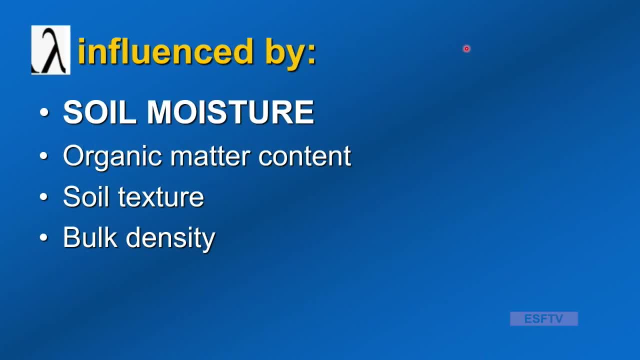 but you'll see it in both. So if you look at the last edition of the text, you'll see it as K And if you look at the current edition, which most of us have, you'll see it as lambda. So lambda is an important number, right? It expresses a flux, it expresses a rate. 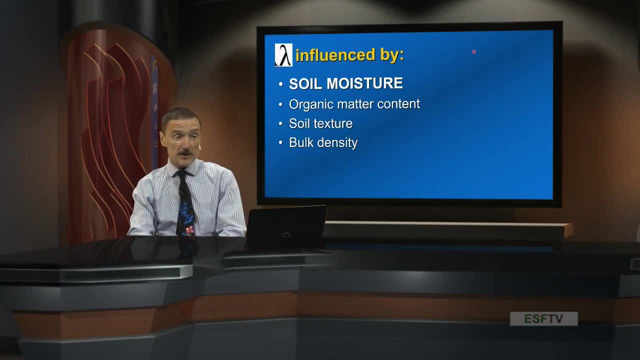 And so what influences lambda, So lambda, So the big one in capital letters here: soil moisture. okay, that's the numero uno factor influencing heat flux in soil, this hydraulic, not hydraulic, this thermal conductivity. Now, once we account for moisture, there are some other factors. 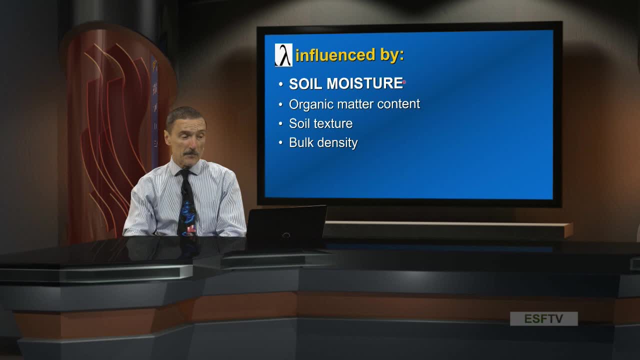 and moisture soil variety. I put in big caps, But then we get down to organic matter content. we get down to soil texture and bulk density. So very similar to the things that affect water flow. okay, And now we'll look at this from the effect. 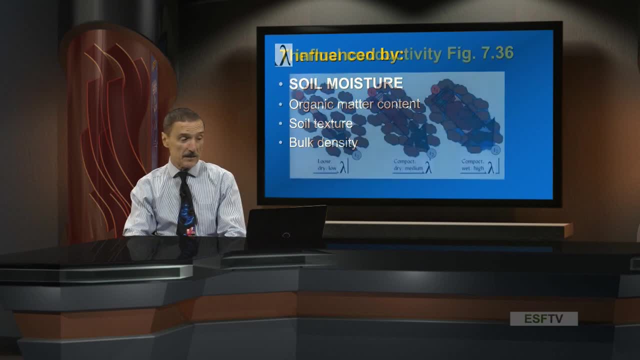 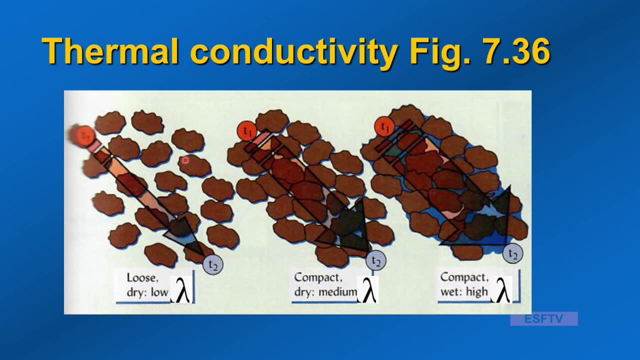 the impact on the flux of energy And it's kind of nicely summarized in this piece in the book, in figure 736.. And here we have lambda, and so in the old one it's K, in the new edition. So you'll see the new edition, these nice colors. the older edition is the greens and the green shades. 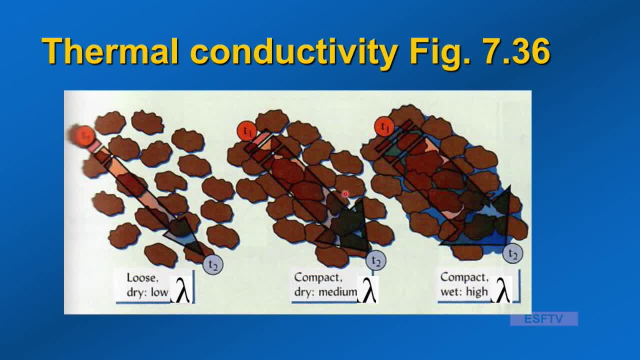 so the same basic picture, but with a nice color And so low thermal conductivity. And this is it. There's little connection between the particles. a lot of air, A lot of air space and dry soil, And so remember that insulation. 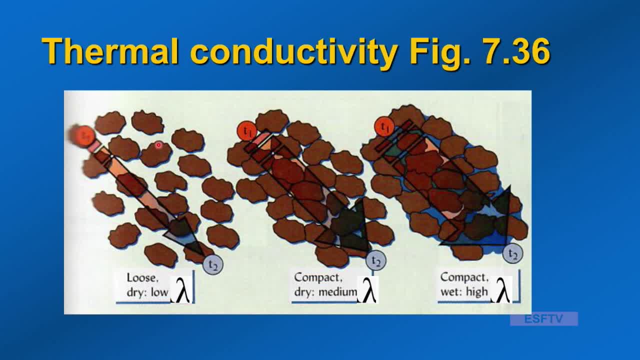 your insulation in your house is largely air spaces. So when you have packed in a lot of air space, you disturb or you make discontinuous the particle connection, And so the rate of transfer of heat energy, the rate of temperature change is very, very slow. 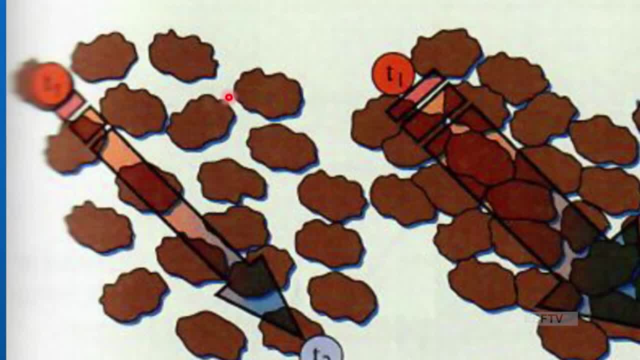 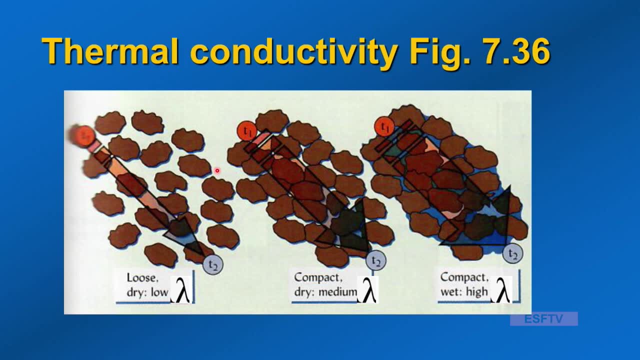 So if you want to slow down the rate of temperature, the rate of heat transfer, just put in a little bit of insulation, add a lot of air. How do we increase that K, that lambda, that thermal flux, thermal conductivity? Well, you increase it by putting the particles closer together, also reducing the air space. 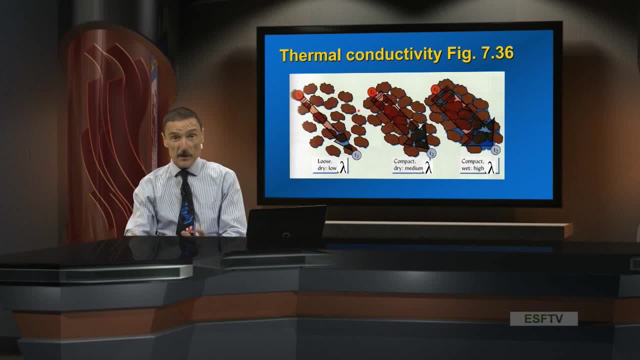 And so when you do that, that increases particle contact and the rate of transfer of energy. the thermal flux increases thermal conductivity. And how do we really increase it? Well, like I said, moisture is big, So this one here over on the right shows a lot of air. 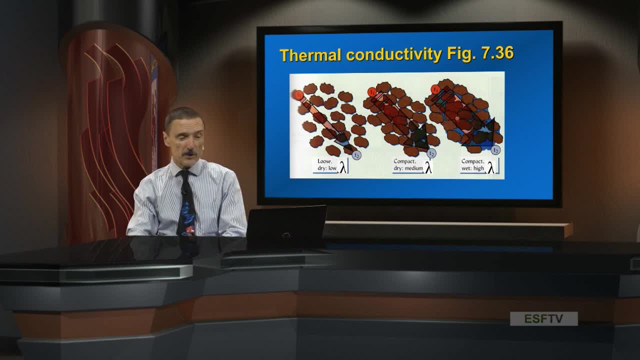 It shows a lot of added moisture. So if you fill all those pores with moisture, all of a sudden you've made a connection and you've driven up the thermal conductivity. So if you think about it, dry more air space, the lower the thermal conductivity. 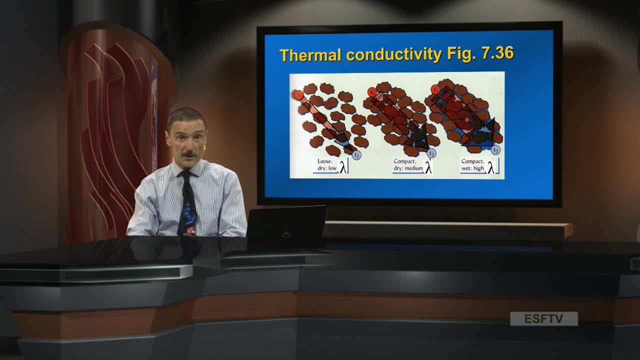 So things like: what about bulk density? So lower bulk density, high total pore space, Lower organic matter means lower organic matter will put things together. A lot of organic matter will keep them apart. So organic matter, bulk density and texture all affect this. 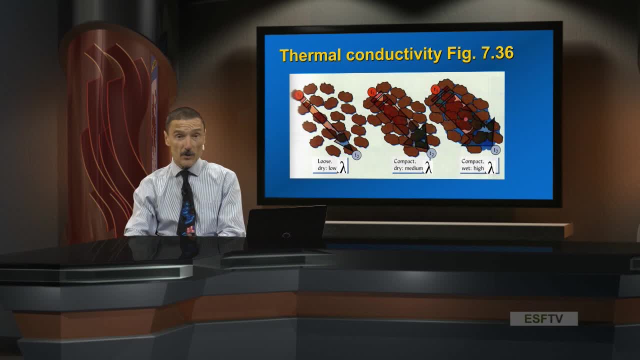 because if you have more air-filled pore space, you have a lower rate of thermal conductivity. Throw in the moisture, pour in the water. all bets are off. Now you're connecting the particles by water and you have a nice high. 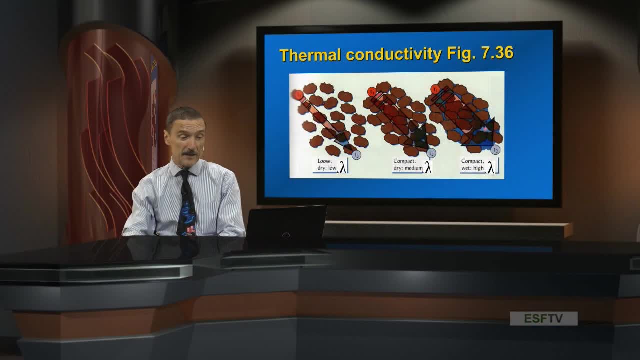 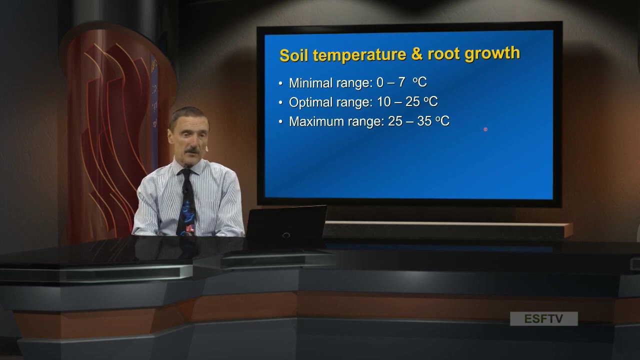 a higher- I don't know if I can say nice, but a higher- thermal conductivity, And that's a pretty good summary of those three factors and kind of integrated in this diagram 7.36.. Soil temperature and root growth. So now we'll think about what this means for the biota. 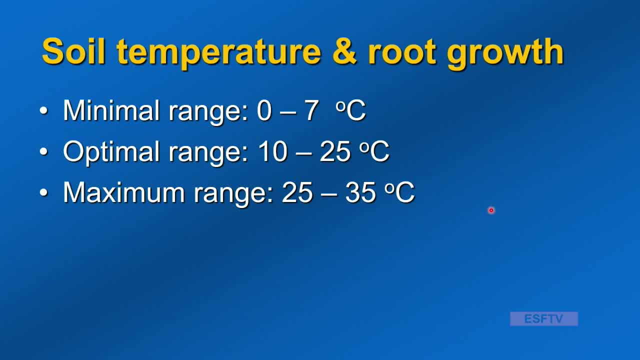 And so there's a range, and in most of our northern species this was from some Norway spruce and some northern hardwoods. these data are actually for Norway spruce seedlings. about 10 to 25 C is the optimal, The minimal range 0 to 7.. And the maximum range 25 to 35.. 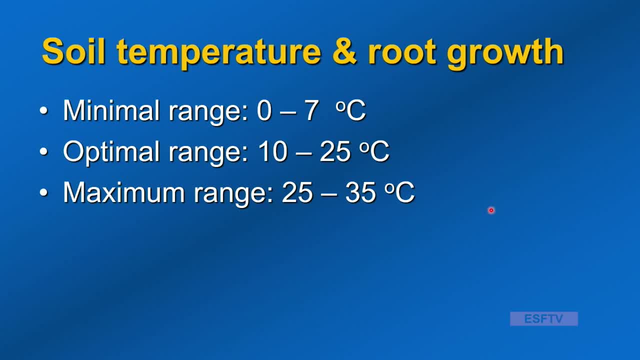 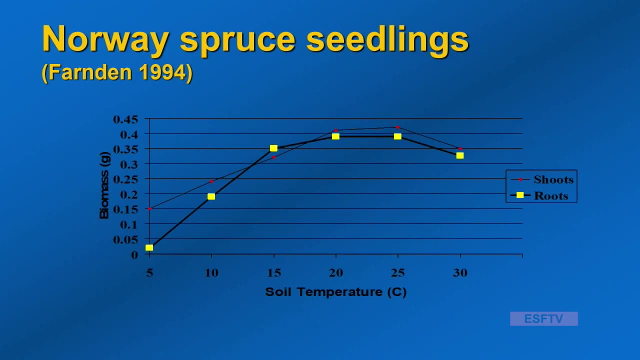 So once you get up to these high temperatures, you're really starting to fry in. You're going to have a real negative impact. All of a sudden you're driving respiration to the point where just all the carbon is used up and soon you denature enzymes and the system breaks down. 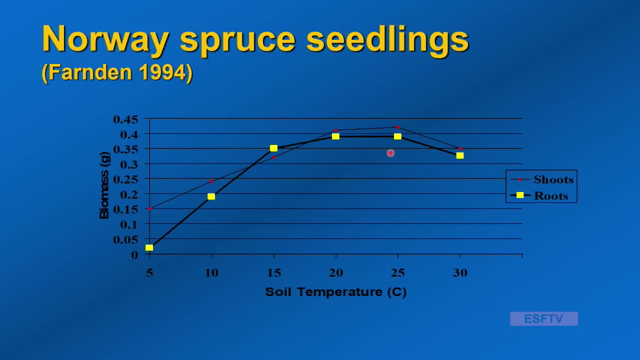 Here's a picture of that. This is out of a publication. a Canadian publication Farnden's some of his work with nursery seedlings, And here we have Norway spruce, and it illustrates these ideas with some actual data. And here we have roots, of course, and shoots. 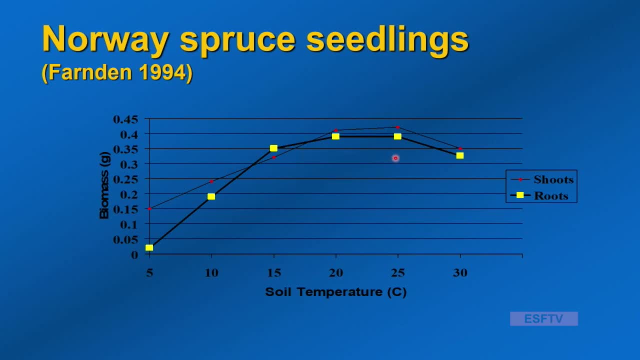 And you can see in that optimal range here the range is not too different from what we just cited. The maximum range is starting to die as you hit past 30 degrees C And the minimum range is 0 to 7.. So you remember this number: 5 degrees C. 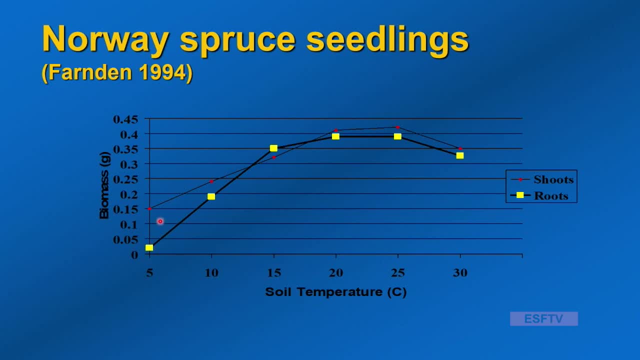 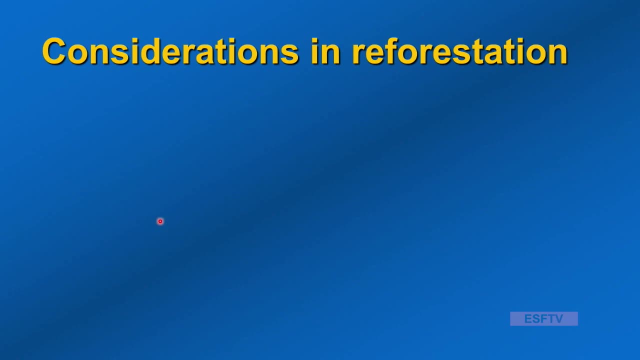 This 5 degrees C. it's kind of smack dab in that middle that idea of biological zero. So this has some applications and implications for reforestation, for planting. We do a lot of planting and many times after a harvest in conifer stands, we'll replant. 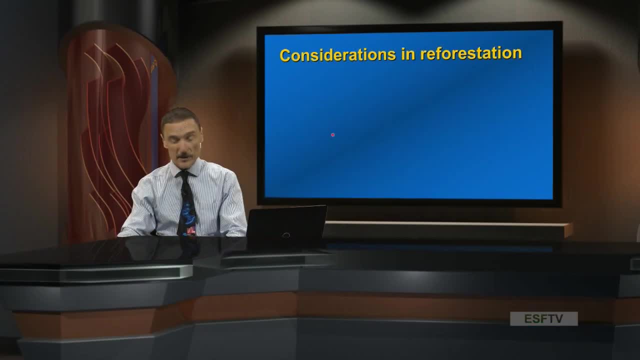 Of course here in the Northeast we don't do that. We have a lot of nice natural regeneration, So we usually rely on natural regeneration- hardwoods. But in many parts of the world we have production forestry and plantation forestry. The planting is key. 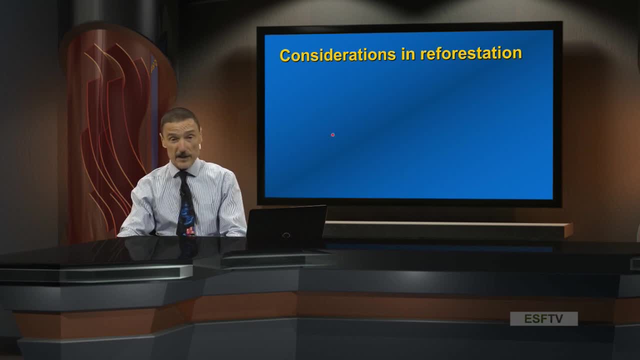 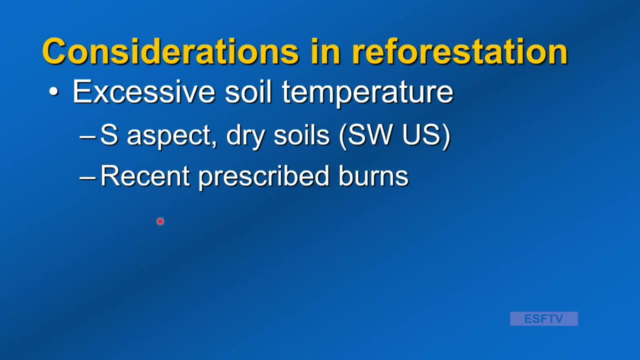 And so we consider soil temperature in our reforestation efforts because it has an impact. And so where does soil temperature get a little bit out of hand? Does it get a little bit out of hand or a little too high? Well, we look in the Southwest, in the western United States. 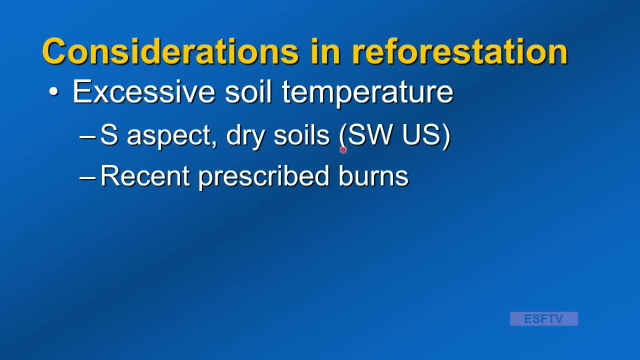 in south aspects and dry soils. So soil temperature can become negative and we have to kind of mitigate against that Prescribed burns. there's a lot of prescribed burns in some of these systems and that darkens the soil and so that can elevate the temperature. 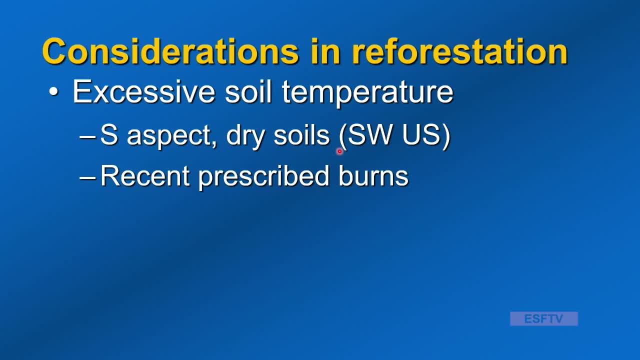 So there are some practical implications of temperature in terms of reforestation. when you're trying to plant things, There's the other end of that: too cold, The deficient soil temperature, not warm enough to get things growing rapidly enough to make those seedlings get through and get ready for winter. 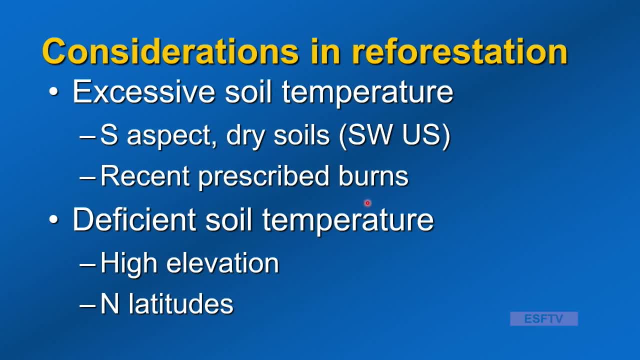 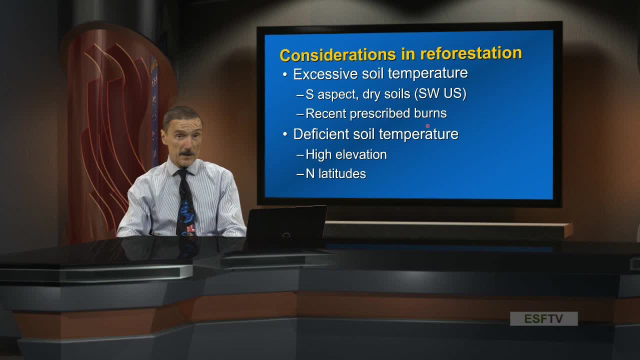 High elevation systems, low soil temperatures, Northern latitudes and then low temperature becomes an issue. So we have high temperatures where in drier areas that can become an issue, Low temperatures in the more northern latitudes and the higher elevations. So that's part of the implications of soil temperature. 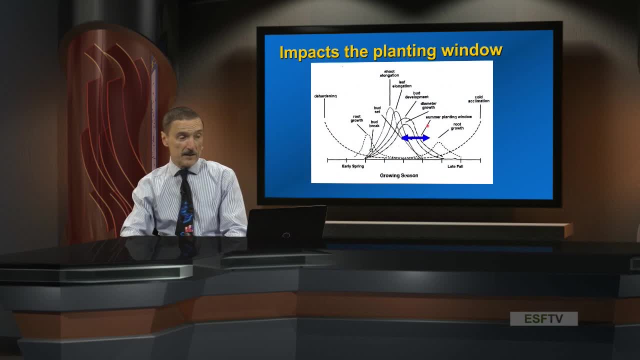 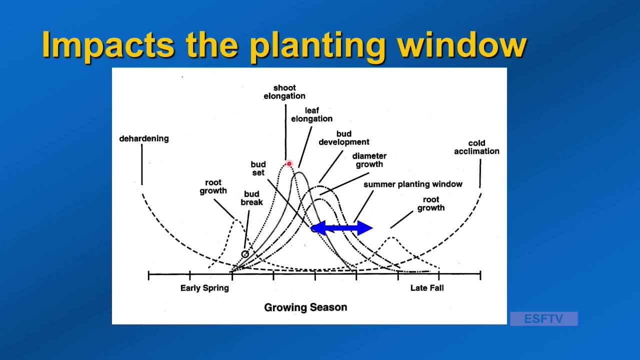 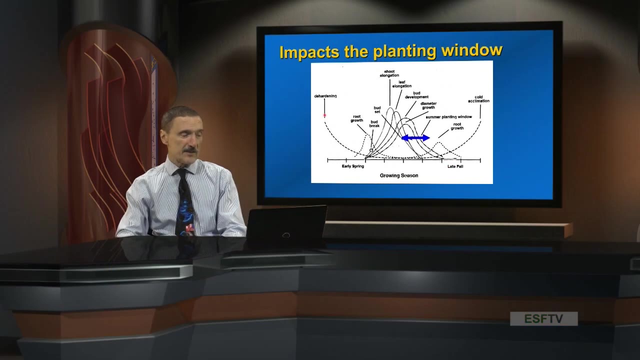 on trying to reforest and regenerate these systems. Here's a nice little picture that shows the planting window on soil temperature. So this shows a variety of phenological development and this is the growing season, early spring to late fall, And in the early spring these seedlings and the trees are coming out. 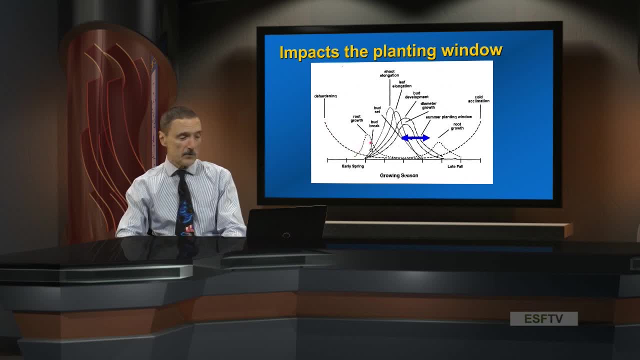 they're de-hardening. All of a sudden they get this pulse of root growth in this early spring and as that root growth slows down, the diameter growth and the above-ground growth takes off. So you see, at the same time, root growth slowing down. 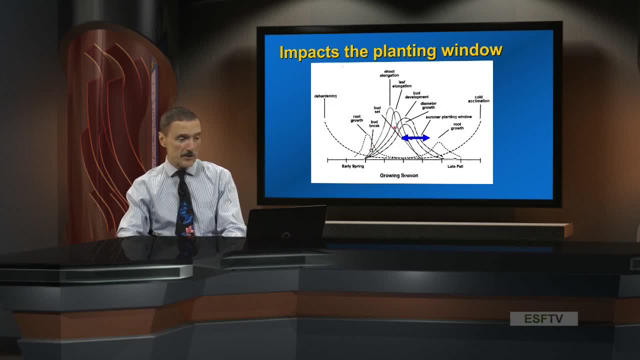 elongation of shoots, elongation of leaves and buds, starting to increase greatly, And then diameter growth and height growth, And so diameter growth and then diameter growth peaks and drops down as we get towards mid-season, mid-summer, going into the fall. 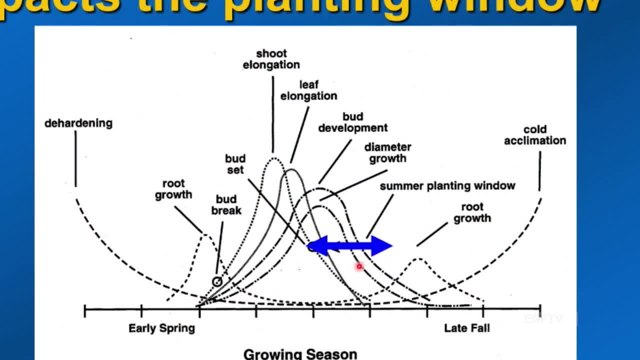 And so where is the optimum place, the optimum planting window? And it's here, just as you come off of the shoot, elongation slowing down, root growth is heating up, And all the way down to late fall where root growth you just want to hit this. 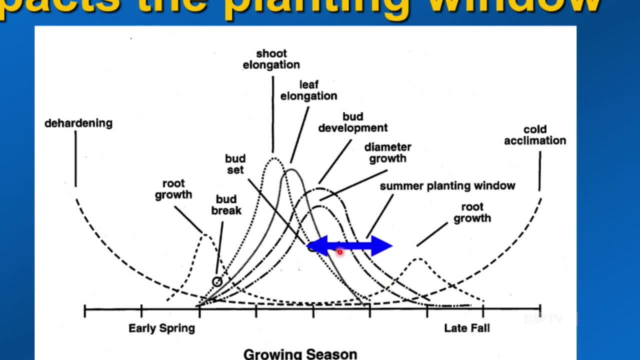 just before you get this next pulse of root growth. So soil temperature is a big driver of this, and so it gives us a window of planting for when we reforest. So this is a practical implication, a practical application of the soil temperature ideas. 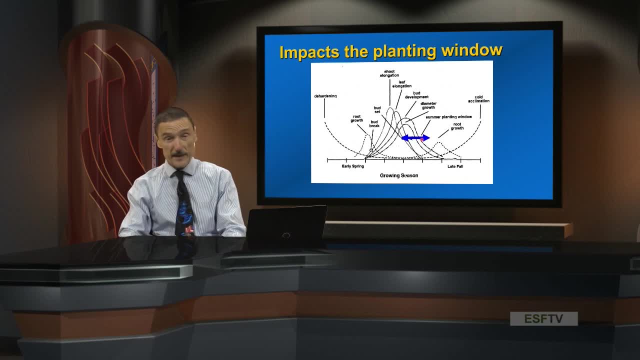 Pretty neat. Of course we don't plant many conifer stands anymore in the northeast really, but where's the big planting? We plant a lot in the southeast. We're doing all this work for labole and pine, our pulp basket, and in the northwest. 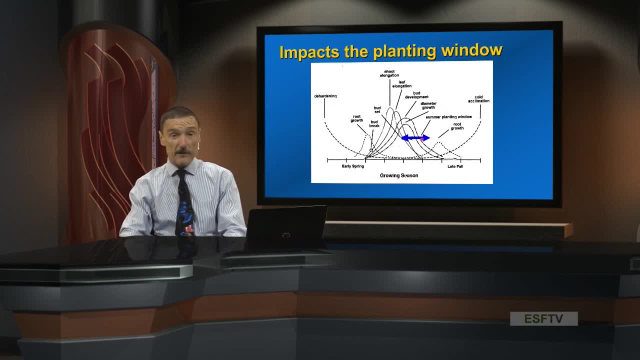 a lot of planting and culture of Douglas fir and various other places in the world, And so for us the planting window is a little wider. right, because we have a little longer season, But in more limited environments you go way up north, it narrows. 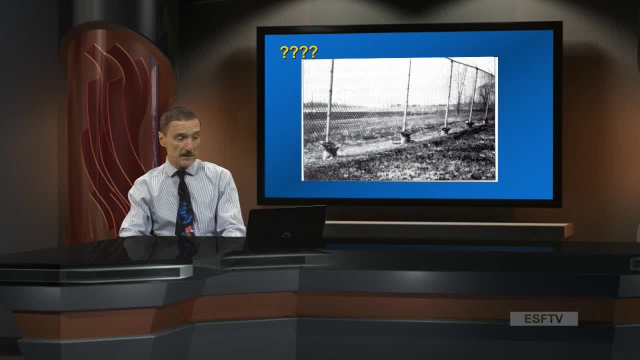 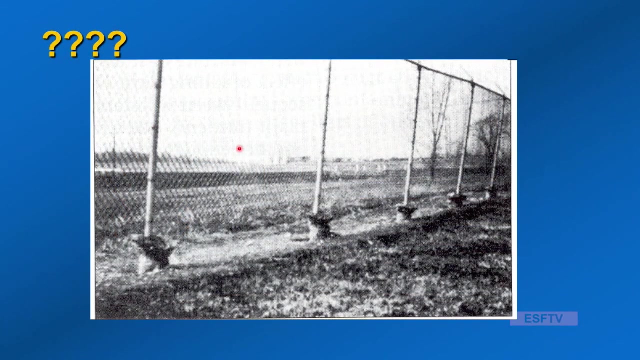 You go into the drier area, it narrows. So that's some pretty neat stuff in terms of practical applications of understanding soil temperature, And there's some more neat stuff, And so I have a picture here, And so what am I showing here? 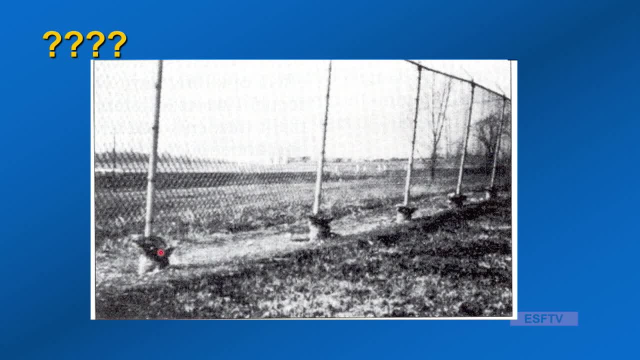 I show you some fence posts and all of a sudden, these fence posts look like they're not where they belong. right, They're elevated. You see these little spots here, And so what's going on here? This is a fantastic example of frost heaving. 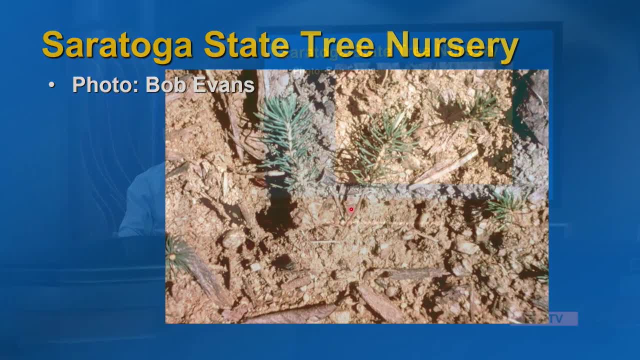 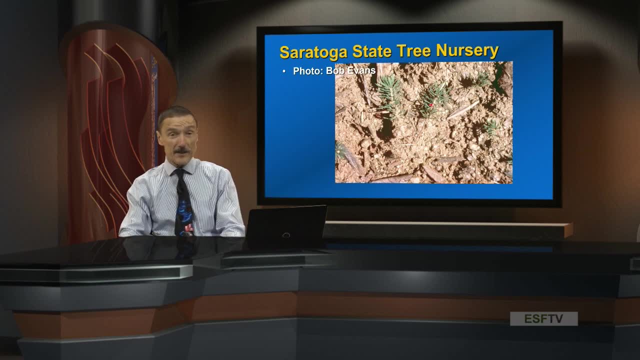 So frost heaving disturbs and physically moves things into places, that it hurts infrastructure And if you're running nursery seedlings and you get frost heaving, you've lost your crop. So frost heaving is a big issue, can be a big issue in forest nurseries. 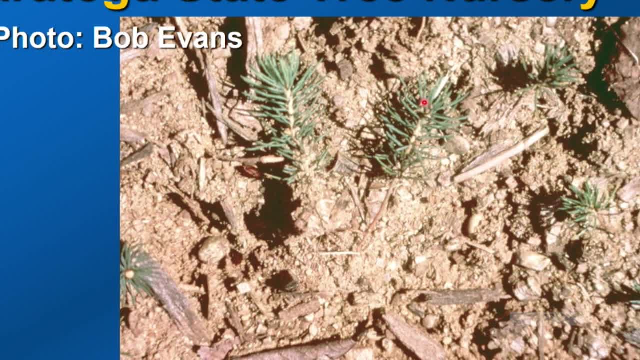 This picture here from Bob Evans, the Saratoga State Tree Nursery. If you take the Advanced Forest Soils test this spring, we make a full-day field trip to this, so it's kind of cool. You can do that FOR 535.. 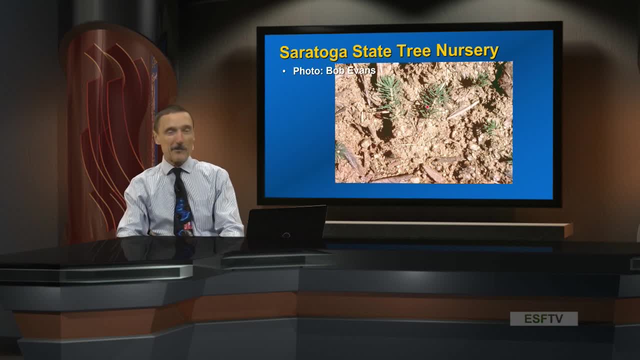 Here's my plug. Here's my plug for the spring course and it's a pretty neat course. So think about it, Look it up in the catalog and ask me about it and I'll say, yeah, take my course, It's cool. 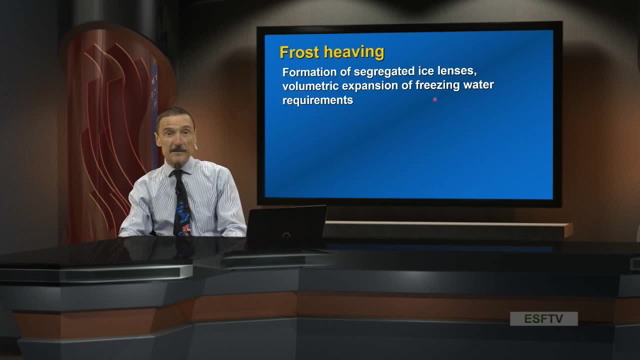 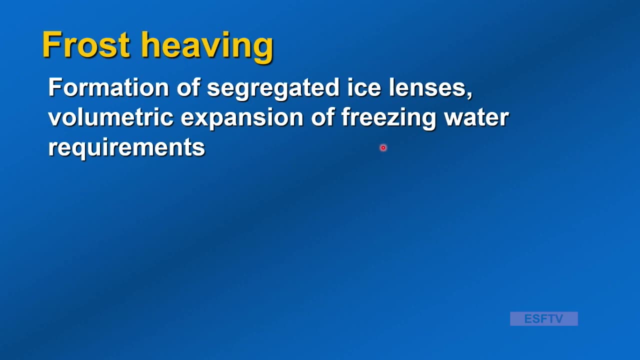 So what is frost heaving? We need to kind of talk about it, maybe define it. And so how would we define it? Well, probably a concise way to do that is to talk about how it's formed and what it does. And so frost heaving. 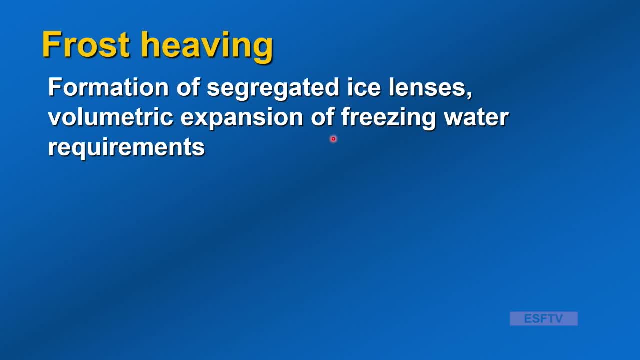 it's the formation of segregated ice lenses, right segregated ice lenses, individual lenses growing in pieces. And what happens when ice freezes? when water freezes, You get a volumetric expansion and so an increase in volume, And this results in shifting. 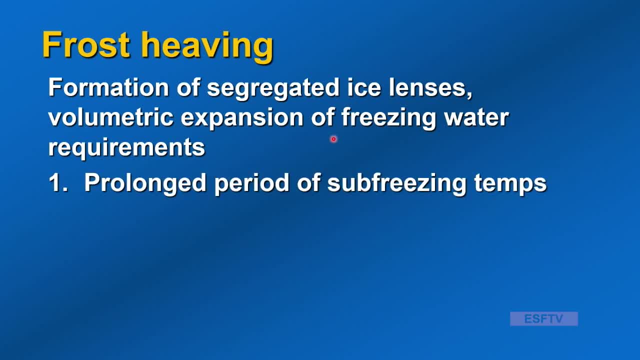 and so this essentially describes frost heaving. So to get that, there are three requirements. First, there's the prolonged period of sub-freezing temperatures. You've got to get down to those lower temperatures, And they have to be for a bit of a time. So a prolonged period of sub-freezing temperatures. That's the first requirement. Second, there's got to be a source of water. You need to continually expand and grow those ice crystals, And so you can't do that unless there's some source of water. 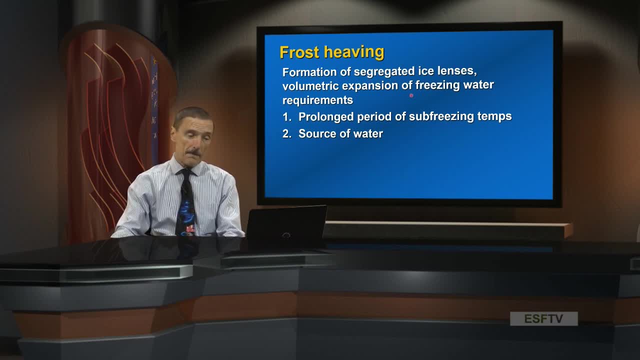 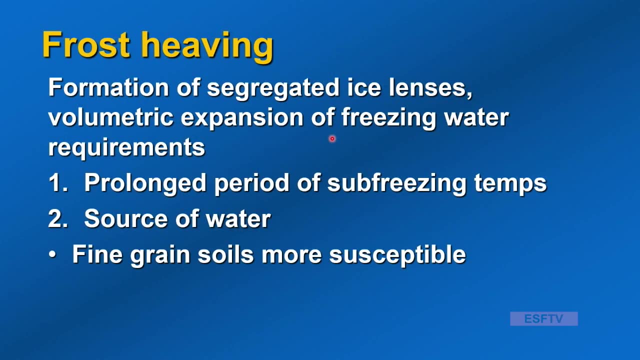 And so that's the second piece of this requirement. So we've got temperatures sub-freezing, We have water, And the next we have a little nuance, And the nuance is the finer-grained soils, finer texture. 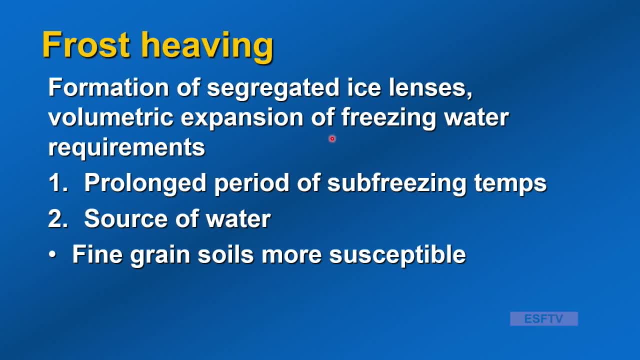 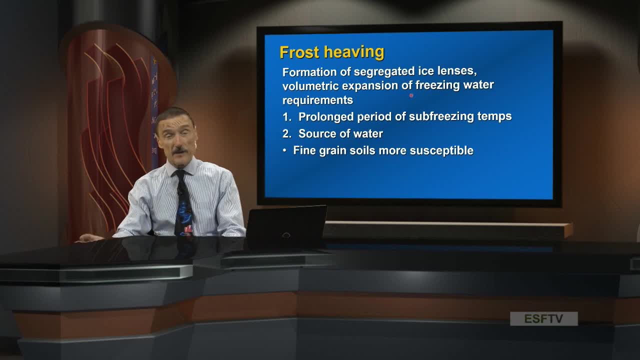 tend to be a little more susceptible. So why would that be? So the finer-grained soils give us a greater chance to move water, a greater rate of unsaturated flow. So we can connect last week with this idea of saturated flow and unsaturated flow and texture. 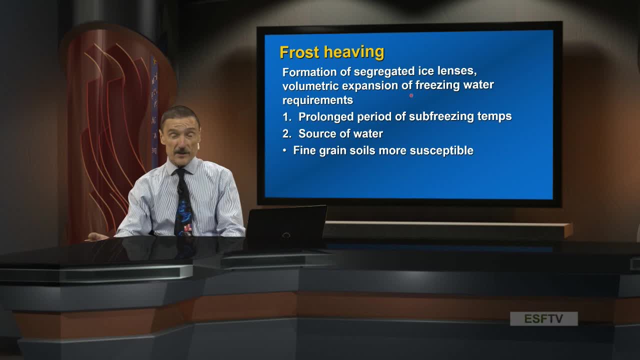 and then think about this as to understand, or think about the nuances of the ease or the increased ability of water to be transported in fine-textured soils compared to coarse-textured soils. So it's not exclusive. You can still get frost-heating. 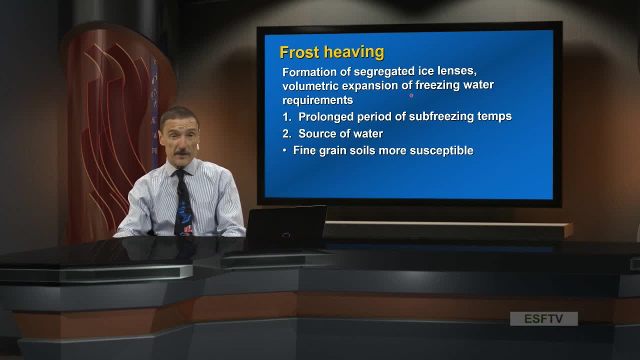 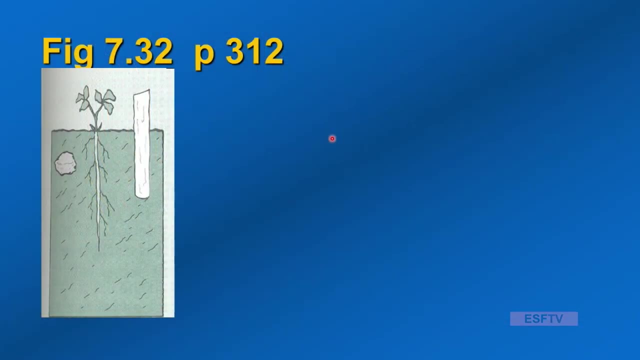 Those soils at the Saratoga Nursery are sandy and loamy sands, but they're much more susceptible as you add more finer textures. Pretty neat. So how about a picture? So the text, the Weil and Brady- has a pretty nice illustration of this. 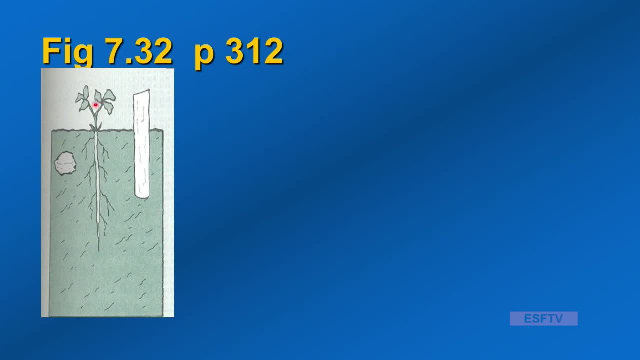 this is 1932.. So it starts out here. here's our plant, a radish plant, a seedling plant, whatever. here's a stone down here and a fence post, and here we are in the fall, and all of a sudden temperatures get cold. 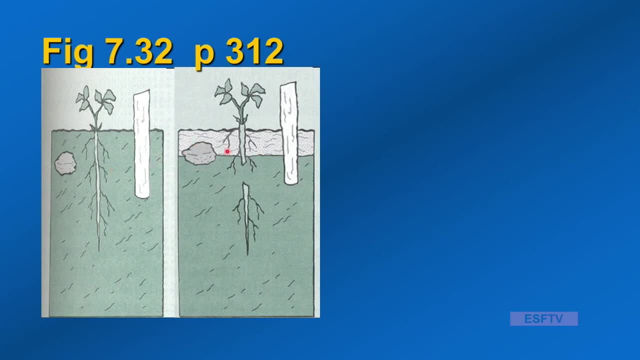 and ice crystals start to accumulate. So these ice crystals grow and coalesce and they shift, and when they shift they increase in volume. and as this is all happening at the surface, there's a little bit of a break here, right? So you have this material being pushed up. 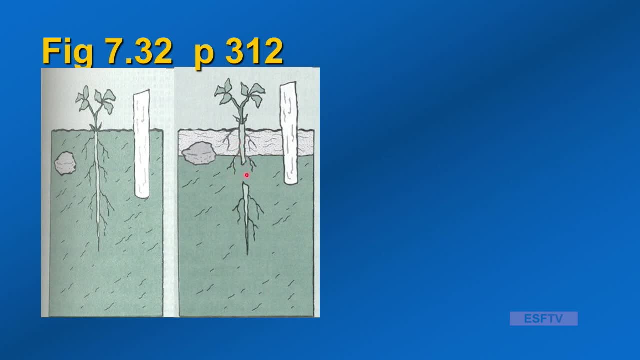 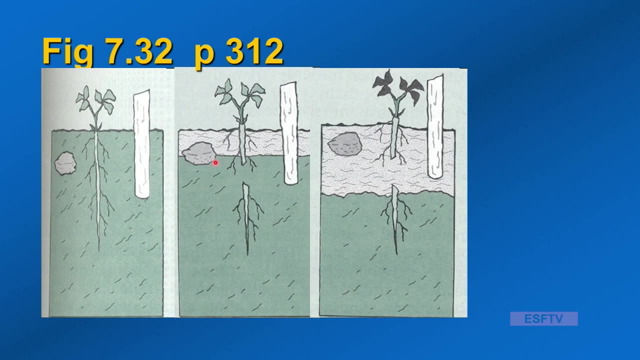 and all of a sudden the plant root here finds itself in a rather precarious position. It's broken. The stone finds itself being pushed up a little bit So that grows. you have a continued source of water and continued transport, and those ice crystals grow. 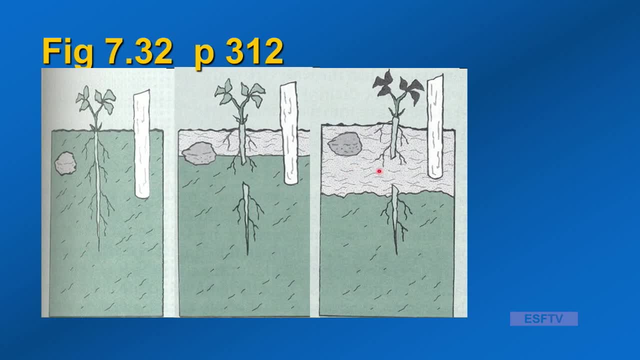 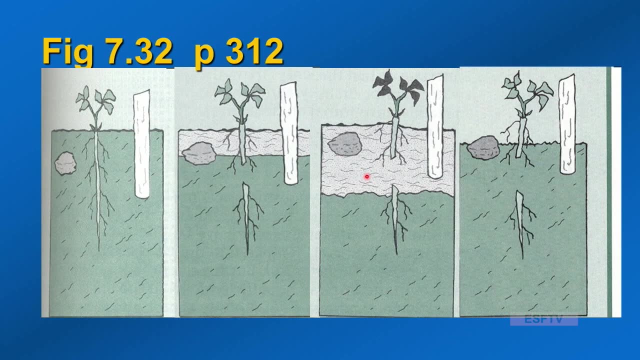 and coalesce even further and this becomes thicker and the displacement is now complete. Eventually it warms up again and you come back from Florida and come back to your house and you've warmed up and you see the stones have been pushed up, the roots are now disconnected. 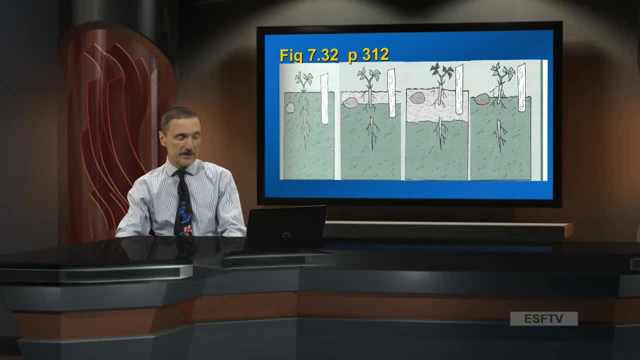 and the fence post is up. So we have this shifting all to this volumetric expansion of water as these ice crystals coalesce And this is the ultimate kind of the nice picture history of an example of frost heaving. So thinking about that, 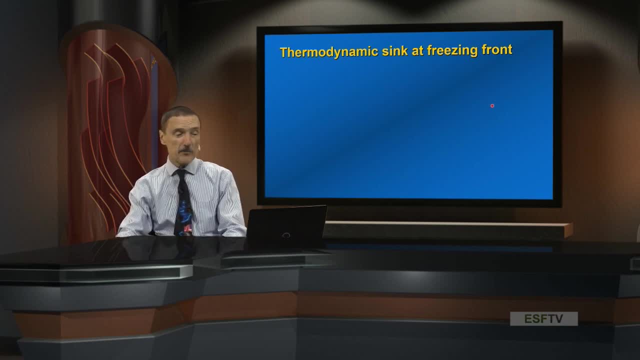 in depth what's going on. There's a thermodynamic sink, So you have this freezing front, right. So we have these water coalescing this freezing front and there's a sink. Water is being drawn to that sink and it's thermodynamically being drawn. 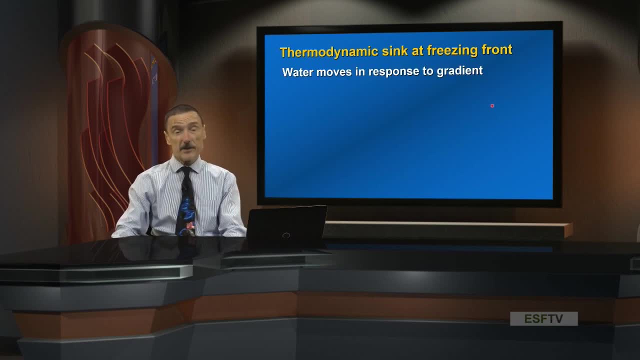 And then there are three gradients. So we discussed last time in water movement in hydraulic and unsaturated conductivity, and saturated conductivity we talked about water moving in response to a gradient And we worked all the way back through potential, And so now we can think about this. 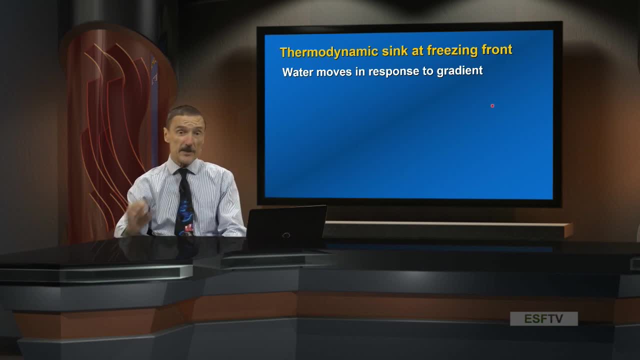 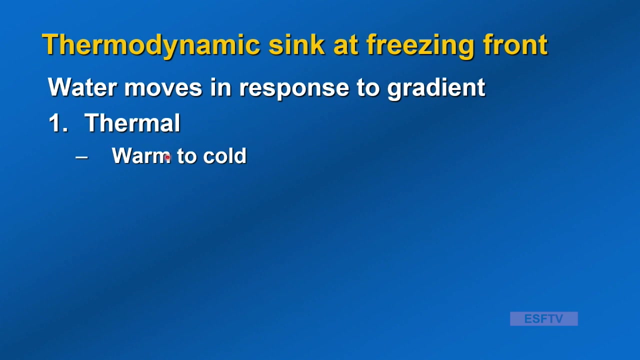 in terms of this freezing area, this little interface as the water freezes and excludes, We have three things going on. So we have a thermal gradient And a thermal gradient so warm to cold. So water is moving from warm to cold And so it's warmer below. 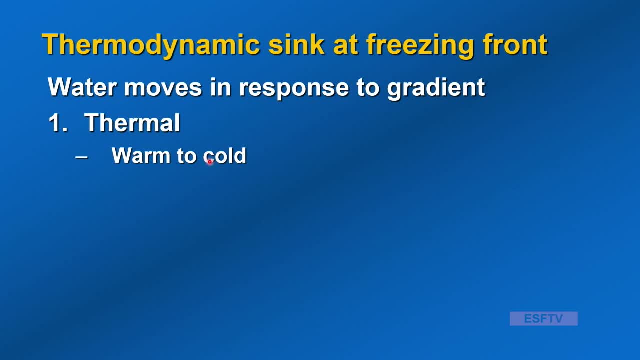 the freezing front is up at the surface and it's colder and water moves toward that freezing front. So this is the thermal gradient drawing water to the freezing front. There's an osmotic gradient, And so remember osmotic gradient, that water moves from areas. 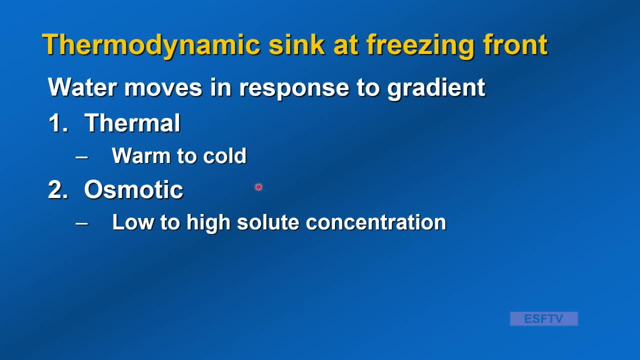 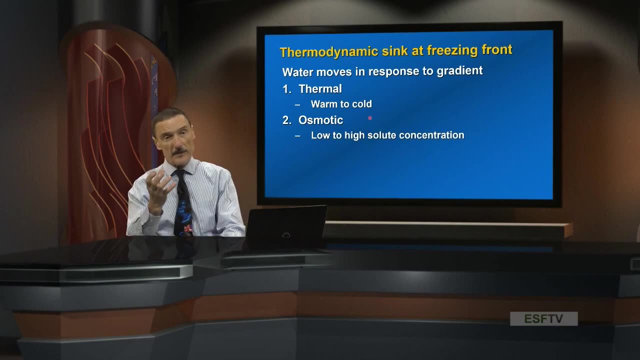 of low concentrations to high concentrations of solute. It moves from clean water, or let's say relatively clean water, to salty water, And so when you're freezing, you're performing, you have this ice and the ice is pushing water out. So what's happening now? 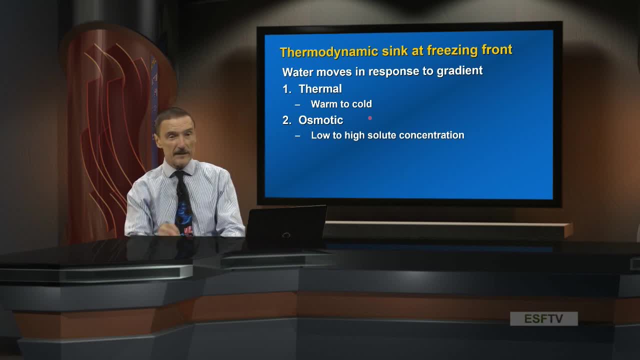 is you have this gradient so that at that freezing front you have an osmotic gradient. Water is tending to move as you're having water and you drop out all the solutes. Water is moving from this low solute concentration in the soil. 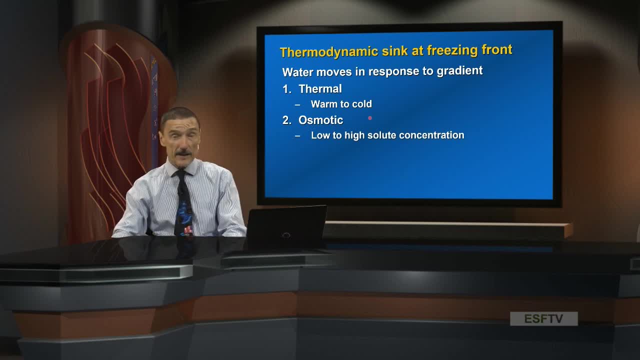 to these solutes being excluded at the freezing front. So two gradients, both working together, and water is moving toward that freezing front. And there's a last one, There's moisture. So the moisture concentration moves from high concentration to low concentration, or from. 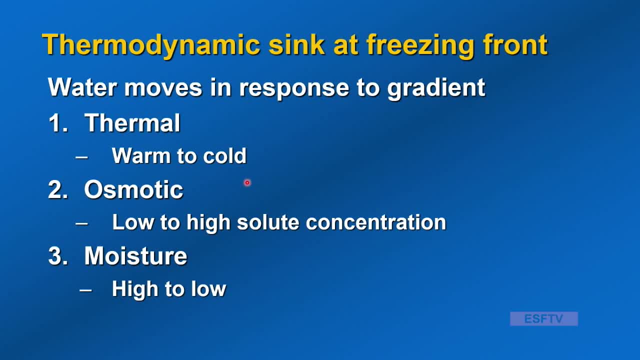 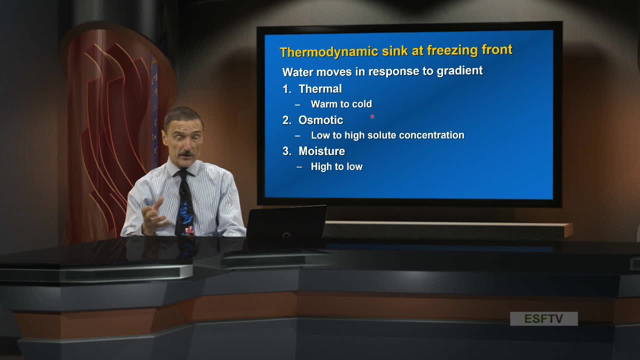 thinking about it the other way, thinking about low potential to high potential. And so, as you're freezing, this freezing front is drawing water through from this moisture gradient, There's more moisture in the soil, You have this continual source and it's being drawn. 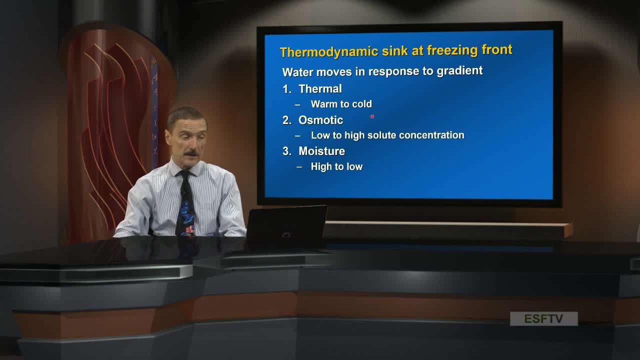 to this desiccated, dehydrated frozen front. So those three pieces- the thermal gradient, the osmotic gradient and the moisture gradient- all drawing water to that freezing front And this ice growth continues And again we've got sub-freezing temperatures. 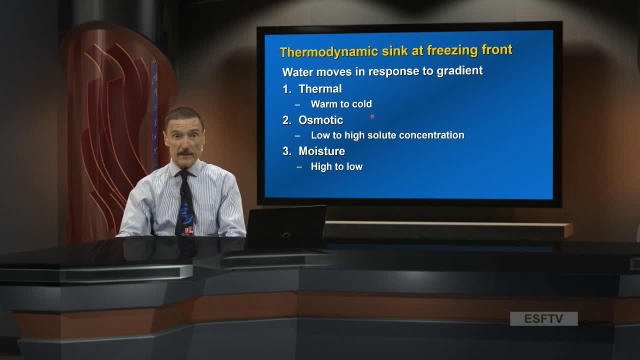 and as well as sub-freezing temperatures, we have a continual supply of water. Cut off the water supply and this process just shuts down Right. Cut off the sub-freezing temperatures and it stops. Nice diagram of that. This was out of a long time ago. 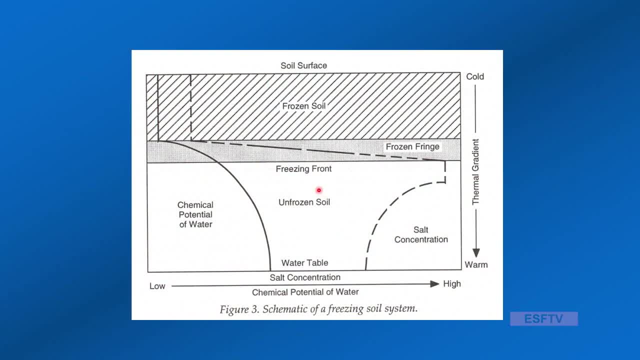 out of a colleague. Giles Marion put something together. He worked for the, for a couple of research organizations, and this was nice, so I borrowed this. I continue to use it. It's dated, But this is a nice illustration. It shows in the hatches. 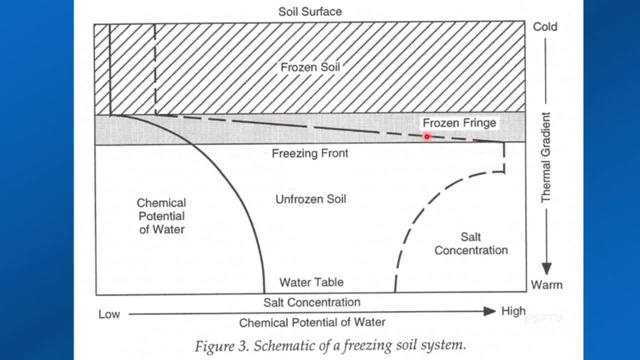 frozen soil up here, And here's the frozen fringe where water is freezing, And so here's unfrozen soil. So we have a temperature gradient. So we're going from warm to cool, Cool to warm, drawing water through. We have a salt concentration gradient. 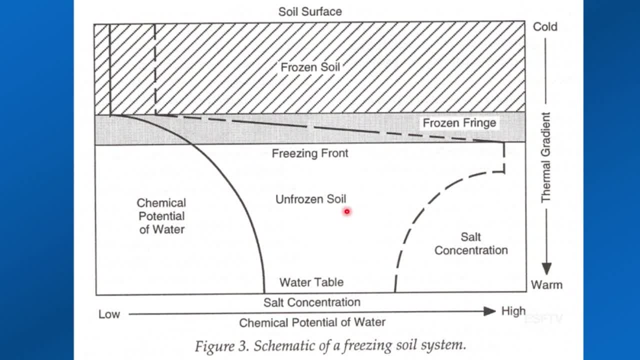 Salt is being squeezed out of here, And so we have higher, we have low potential here, and higher potential here and lower potential here. So this difference in osmotic gradient- relatively unsalty to this frozen fringe- And then the temperature gradient, It's all again. 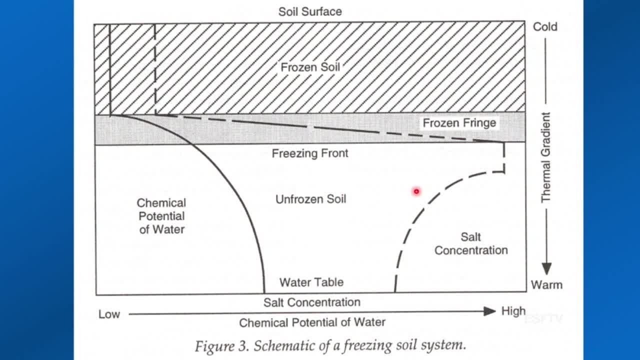 those all working together. So it's kind of neat And this illustrated here. on this axis we see cold to warm- It's cold at the surface, warm going down The potential of water low to high. And as you get towards the, as you get toward the, 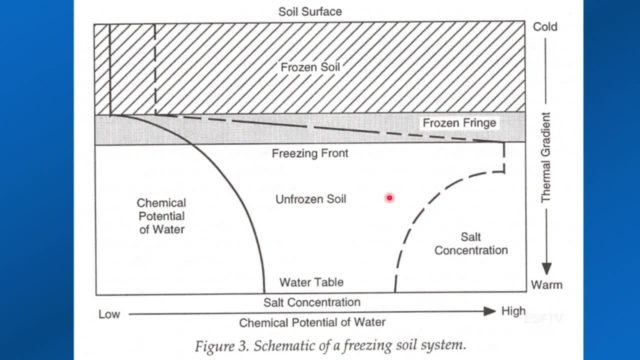 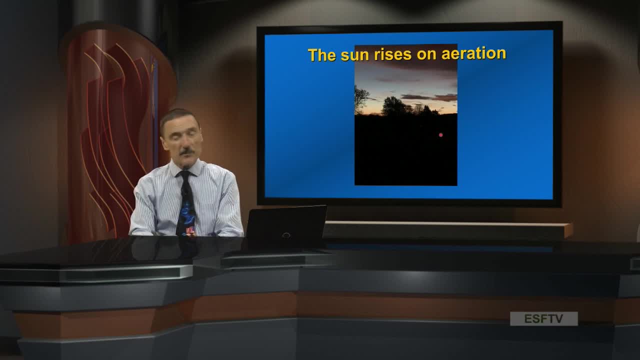 frozen fringe, the potential is reduced, Pretty nice. So that kind of completes our work on soil temperature. It wraps up where we began last week and last Wednesday and finishes it up, And now we begin to talk about soil aeration, And so here's a sunrise. 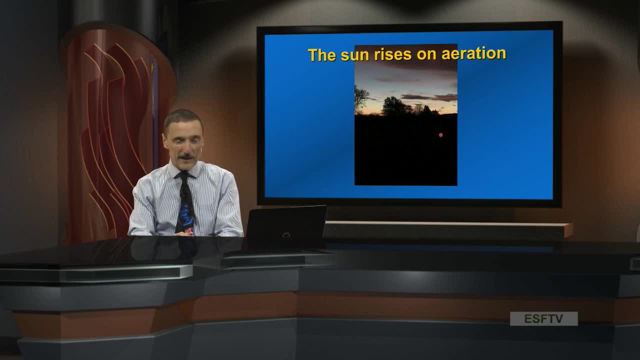 So I took this. I do a do a pretty 21 mile bike ride every morning and just get back around sunrise- And this is just a picture- just not too far from between Marcellus and Skinny Atlas. And so here's our sunrise on aeration. 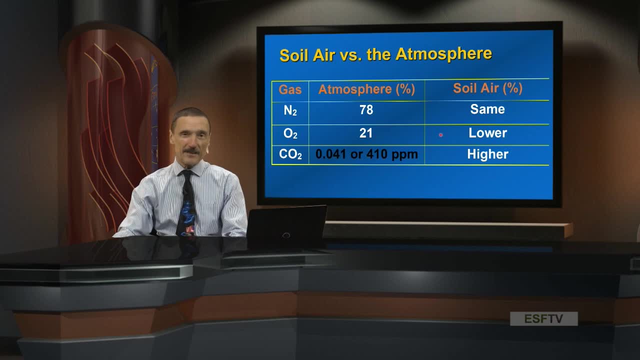 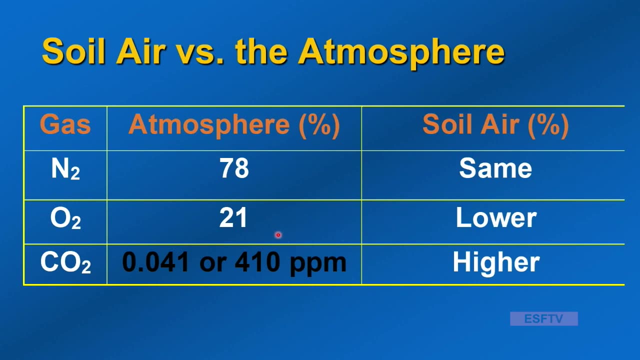 So let's consider first the composition of the atmosphere. What are the three main gases? So nitrogen 78%, Oxygen 21% Carbon dioxide: 410 parts per million Right now I remember it was it was in the low 300s when I was a student. 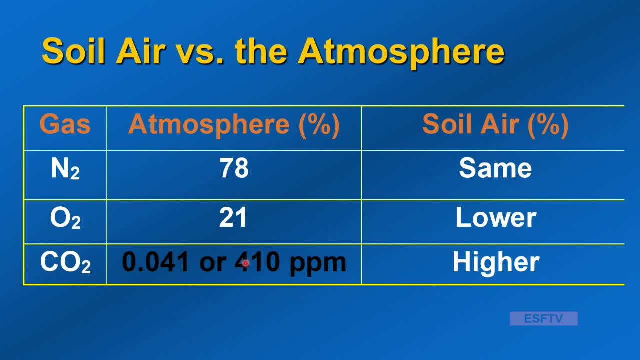 And so never thought it would go up to 400. you know, break 400. And here we are, we've broken 400 ppm, So rather extraordinary times. But so so these are the concentrations of the atmosphere, And so parts per million you can convert to percent. 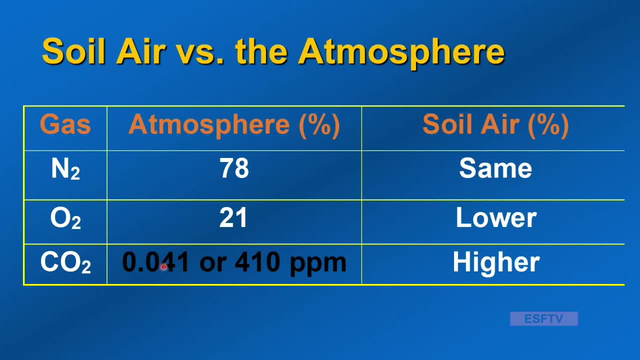 And so this is a percent: 0.041.. And remember this parts per million is parts per 10 to the minus 6.. Right, So you have 0 0 0. And if you look at that, the percent is 0.041%. 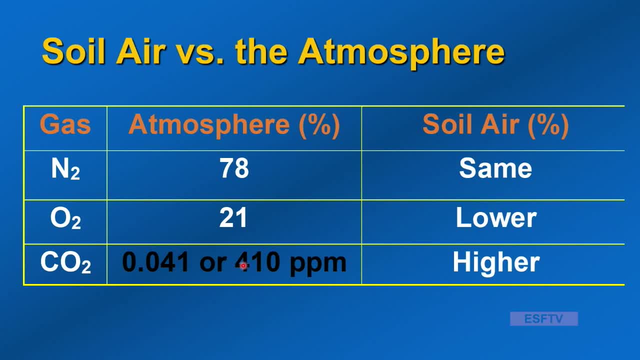 So you should be able to make that conversion. So that's the atmosphere, And let's consider how that's different from the soil air, the soil atmosphere, So nitrogen, is relatively inert. It's the bulk of the. it's the bulk of the volume. 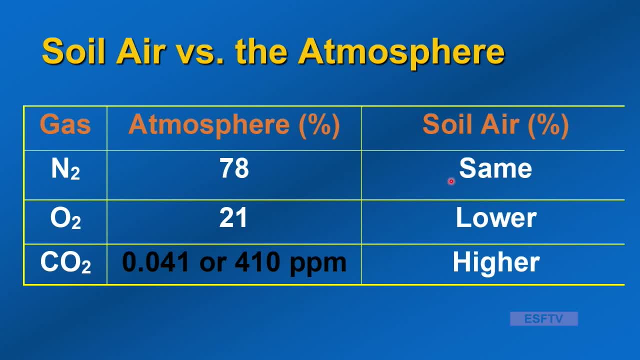 of the gases And it's about the same concentration in soil air. Oxygen in the atmosphere: 21%. It's lower in the soil atmosphere. in the soil atmosphere And we'll see why it's being used up. Carbon dioxide: 410 parts per million. 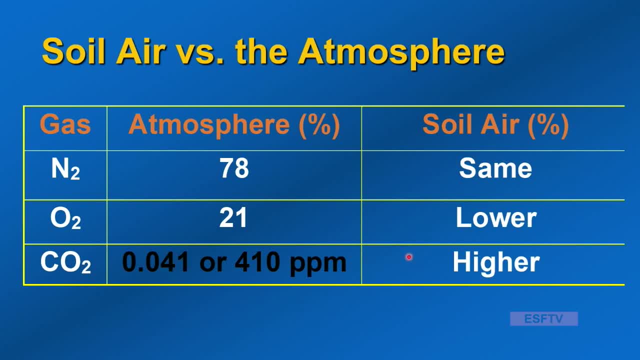 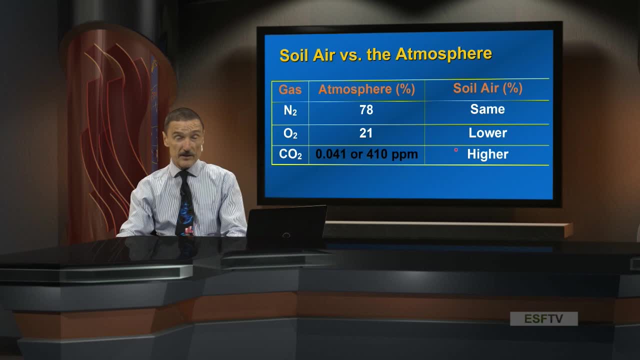 or 0.041%. It's higher in the soil And the how much lower and how much higher. this depends on the degree of aeration. And so now we've got a motivation to think about aeration. We have something to compare to. 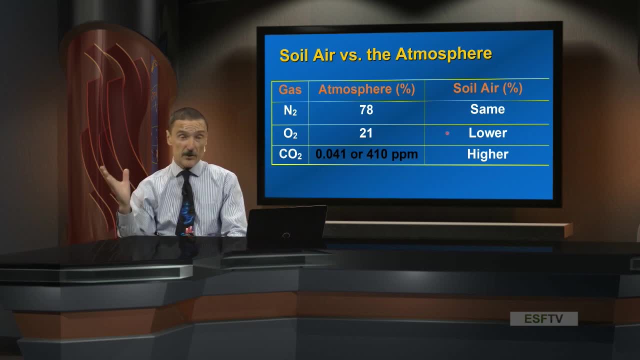 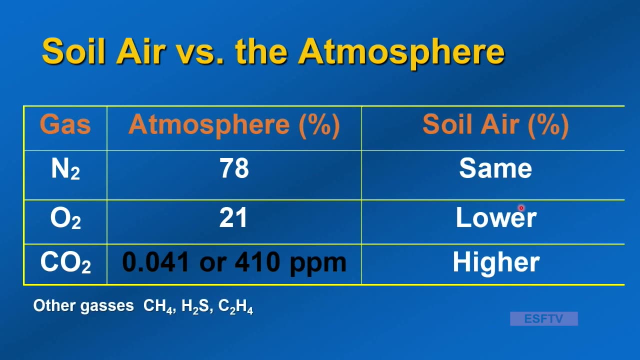 We have the atmosphere, So we can talk about the atmosphere above the soil and the atmosphere within the soil, And so let's continue down that pit, so to speak. So those aren't the only three, There's a lot of other ones. 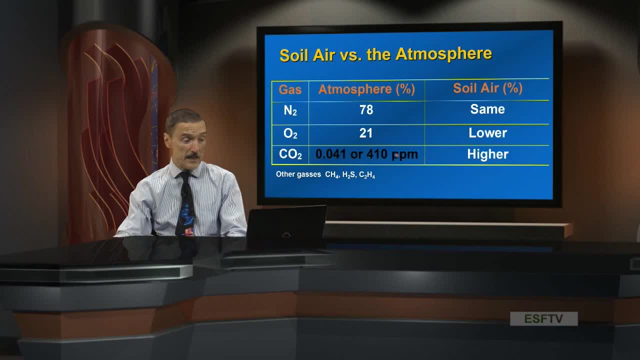 They're small concentrations, Big importance. But methane and hydrogen sulfide and so forth And ethylene, All kinds of pretty cool gases, but in very small concentrations, But not to say they're not important. Methane just way outpowers carbon dioxide. 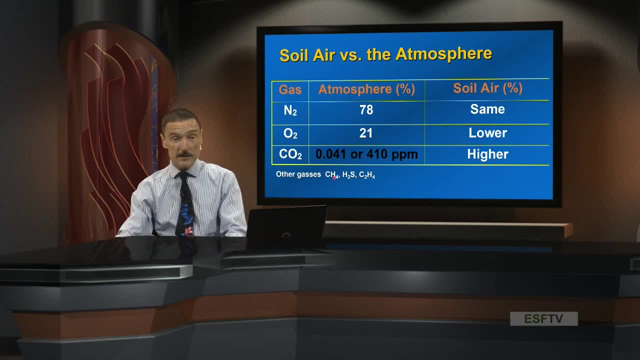 in terms of its impacts on ability to trap heat. So all these are important, But for our purposes, in terms of just thinking about aeration, we'll kind of focus on oxygen and carbon dioxide for now, And the fact that there are lower oxygen concentrations. 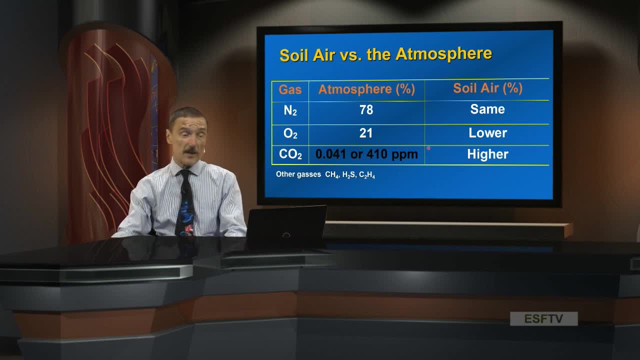 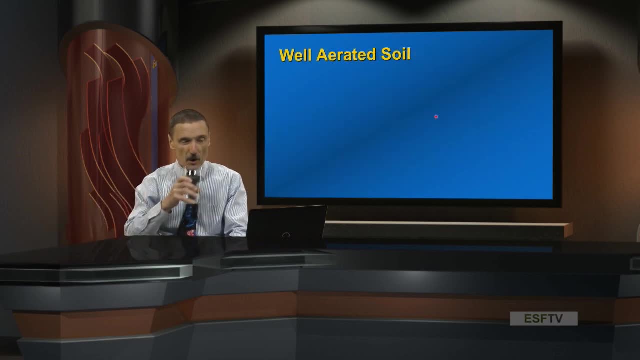 in the soil layer, higher concentrations of carbon dioxide in the soil layer and about the same as nitrogen. So we could ask: what is a well-aerated soil? What do we mean? So the definition helps. So when we're talking about 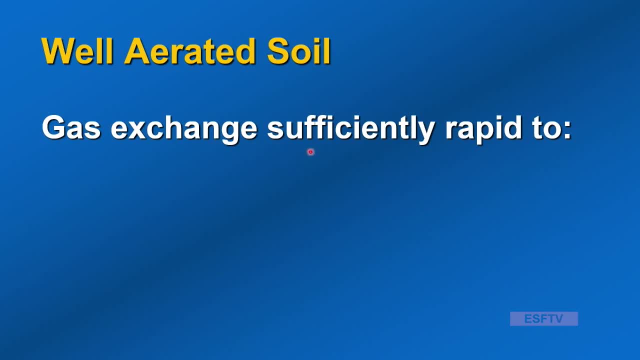 a well-aerated soil- we're talking about gas exchange- sufficiently rapid. It's always like to have these little phrases that kind of lead up. So these are five little words that are quite important: A well-aerated soil, the gas exchange. 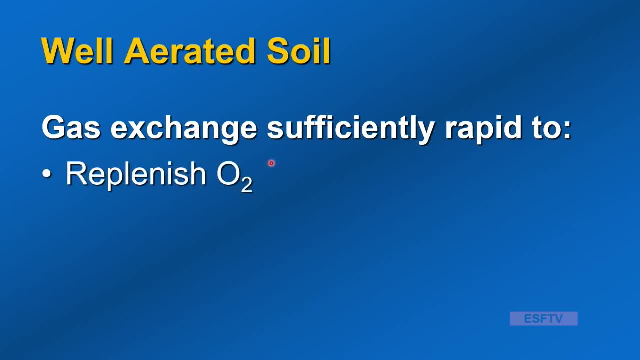 is sufficiently rapid to replenish oxygen. So who's using oxygen? The roots are using it, The organisms are using it, All the aerobic organisms. just has to be replenished or the system kind of comes to a halt or slows down. The other thing you've got to get rid of. 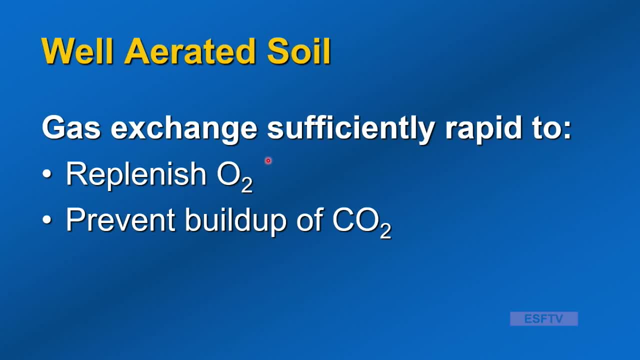 is the gases that are toxic into the aerobic organisms. CO2 is a buildup of that is reduces productivity and actually can lead to some to death, to death and destruction. It slows the system down, So you want to replenish the oxygen. 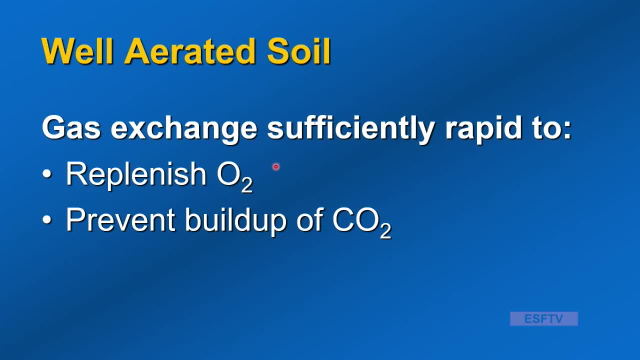 and prevent the buildup of CO2.. So gas exchange has got to be rapid enough to do that. Okay, so that's a well-aerated soil. We have enough oxygen that's keep coming in. We're greening out the CO2.. 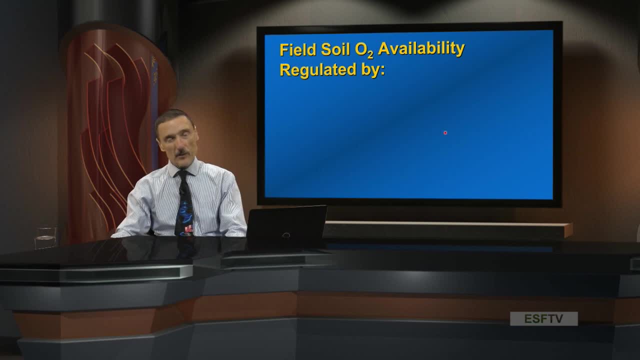 So what we can think of next if we've got a well-aerated soil, what regulates oxygen availability in the soil atmosphere? So who's using it? So the first thing it regulates is how fast you can move it, And air and water. 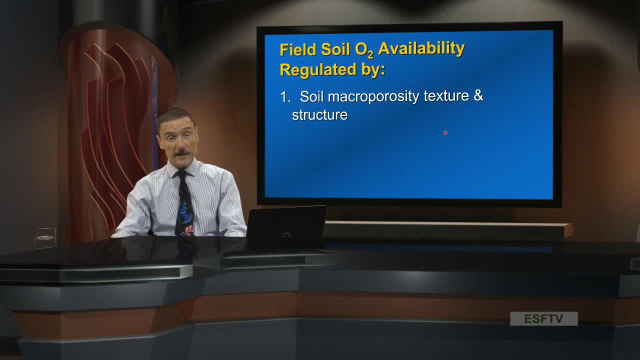 largely water moves through macropores. It's either filled with air or filled with water. So macroporosity, texture and structure- three big ones. So the macro. the more macropores, the greater the chance the water's going to leave under gravity. 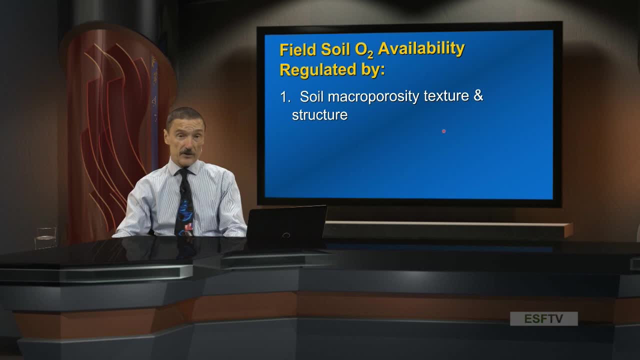 and the better. the aeration, Texture and structure contribute to pore size distribution. We've talked about the impacts of pore size with fine textured clays and small pores and larger proportion of micropores. We've talked about the large proportion of macropores. 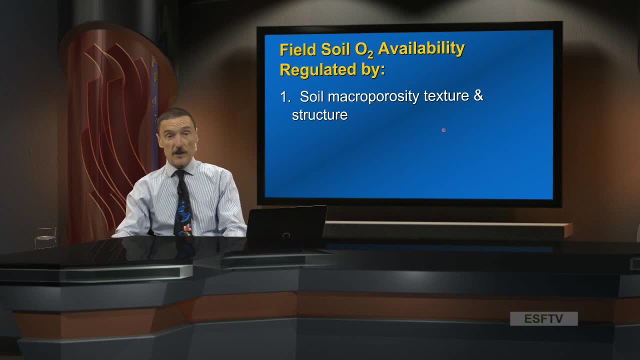 in sandy soil, And we've talked about structure and the improved effect of porosity. macroporosity due to structure- Nice well-developed granular structure- increases macropores. Macropores allow water to drain. Water drains. 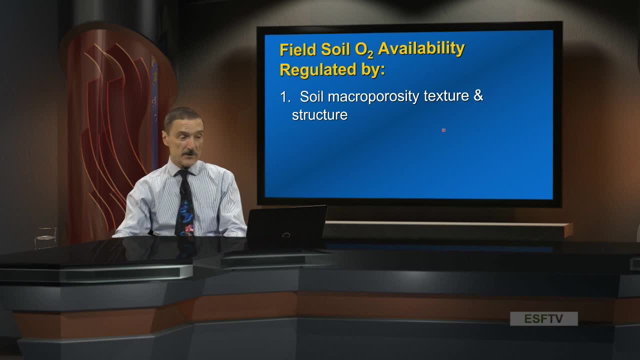 allowing air to move through. So these three factors regulate availability And these are the physical factors, and so we're essentially continuing on our lecture and our ideas about soil physical properties as we translated those into soil water, and now kind of think about what that means for aeration. 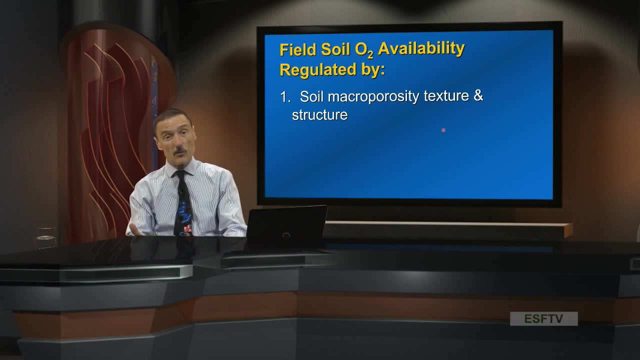 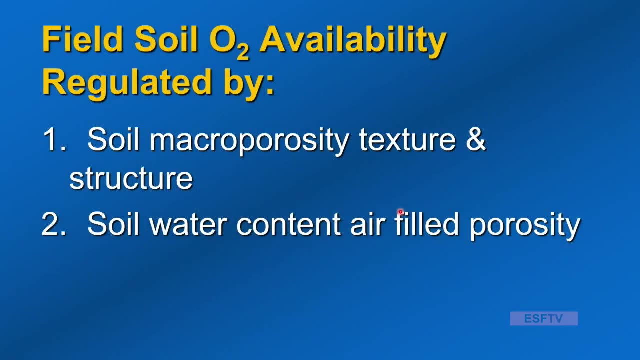 Again, aeration is the other side of water. right, If you have no water in pores, you have a way to move air through, and vice versa. And so the soil, water content, the air-filled porosity, total porosity- how much of that is filled with air? 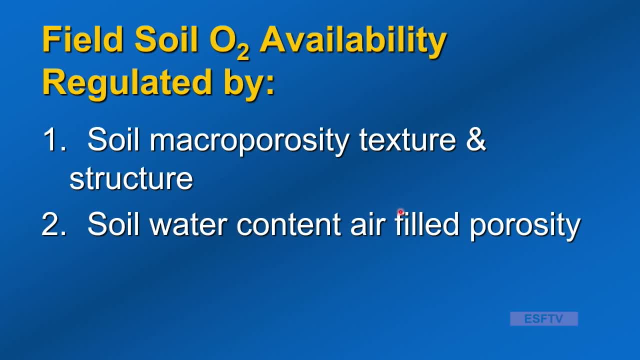 how much is filled with water. So that's going to govern the capacity to make oxygen, move oxygen through as well as move carbon dioxide out. And finally, the users: O2 consumption: Who's using roots? Who's using O2?? 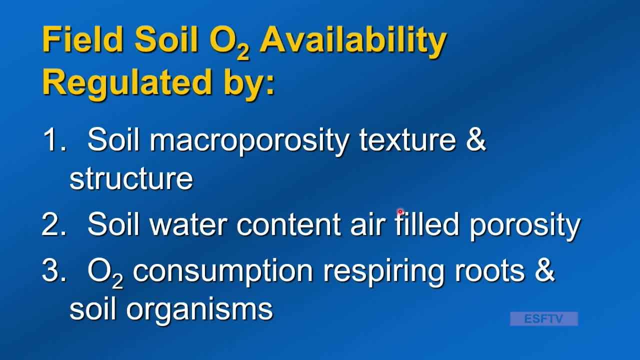 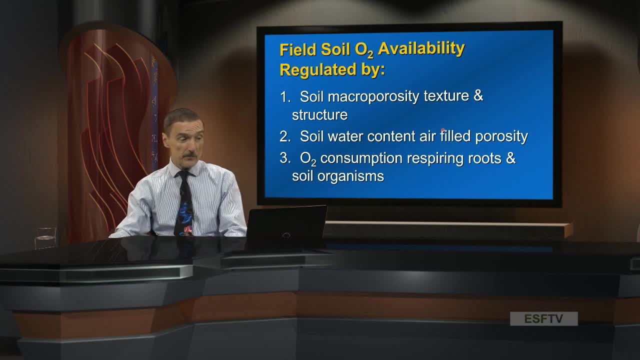 The roots, the soil organisms, all those aerobic organisms that require oxygen to run respiration. they're consuming oxygen. So these are the three, pretty much the three drivers when we think about how do we determine how much oxygen or how do we assess oxygen availability. 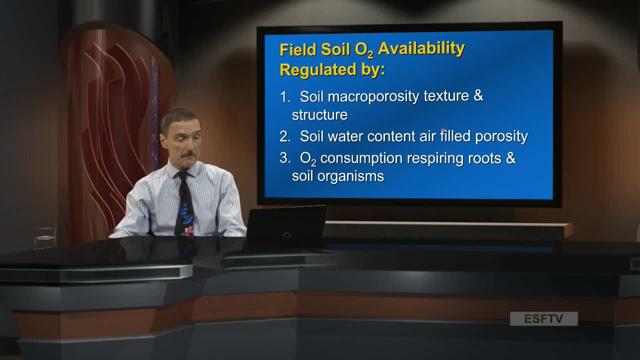 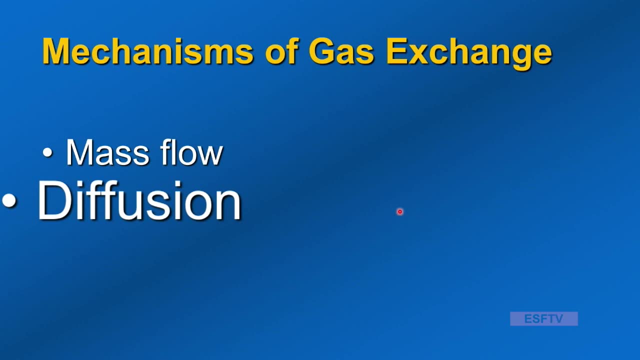 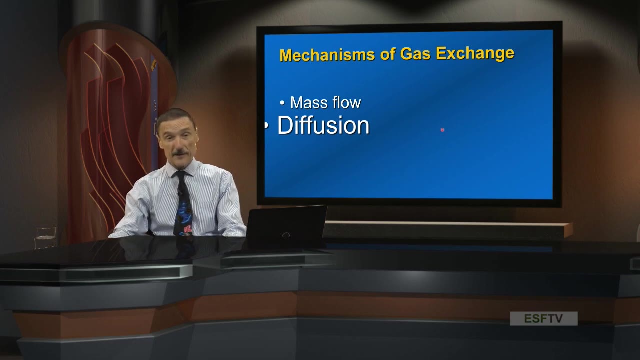 These are the three bigger pieces of that. So that brings us. how does air move into the soil? How does the atmosphere gases, how do they get into the soil, Those fluxes? remember we talked in the beginning about the fluxes of energy, water and gas. 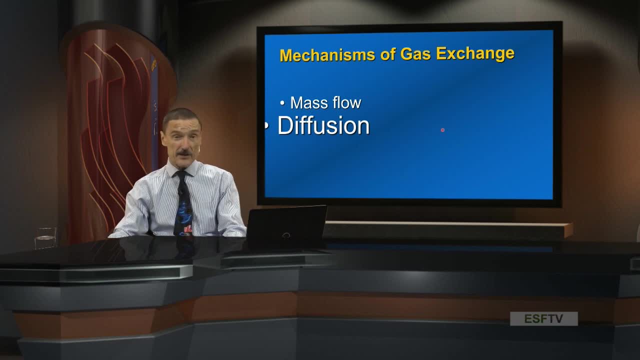 and now we'll focus on the flux of gas in these systems, through this biogeochemical membrane which we call the soil. And there's two ways to do it right. There's mass flow, so simply by air movement. air's 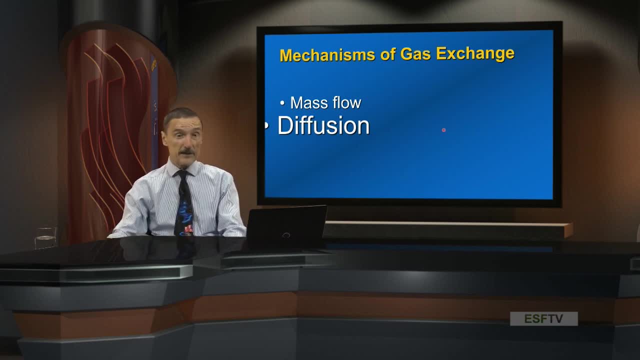 parcels moving around and wind and so forth. And the other way is diffusion. And the primary, the primary mechanism here in soils to move air through soil systems, exchange atmospheric air for soil. atmospheric air is the process of diffusion. Big letters. 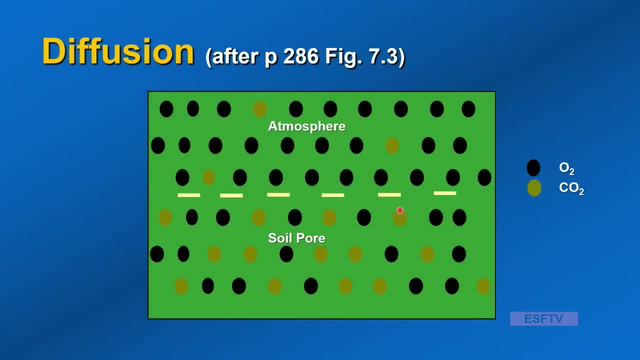 So let's illustrate Diffusion. So remember from your chemistry that diffusion is the movement of a substance against, in response to a gradient, And so this time we're talking about gases in response to a gradient. So this is a little cartoon in the text. 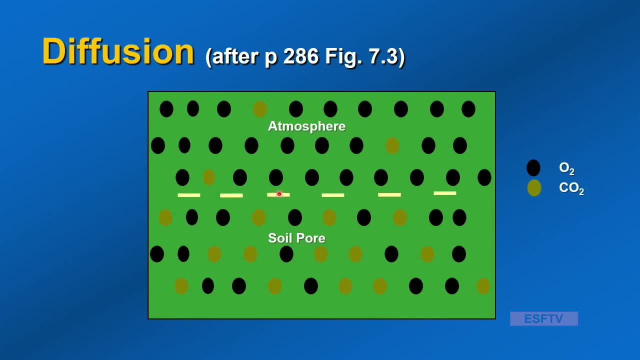 Here we have the atmosphere and the soil pore. Here's the soil-air interface, in these little dotted lines, And here are these soil pores. And so this represents oxygen, is represented by the black relative concentration of black dots and CO2 by the relative concentration. 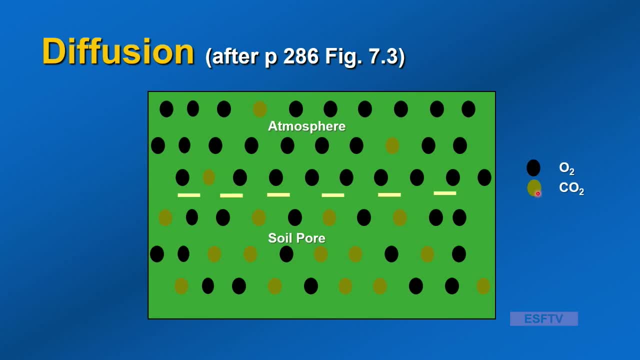 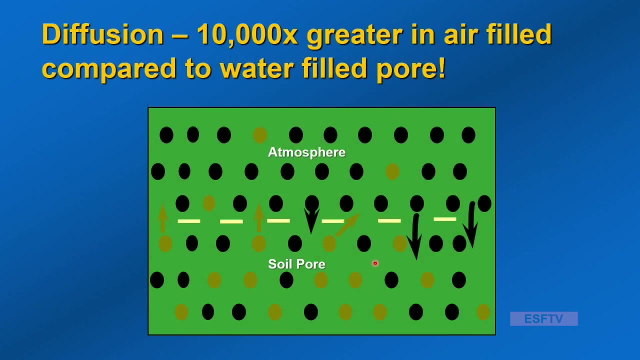 of these lighter, I guess yellowish, 5y6, over 2, I don't know. At any rate, the movement here is in response to a gradient. So where's it going? So here we have carbon dioxide and here we have oxygen. 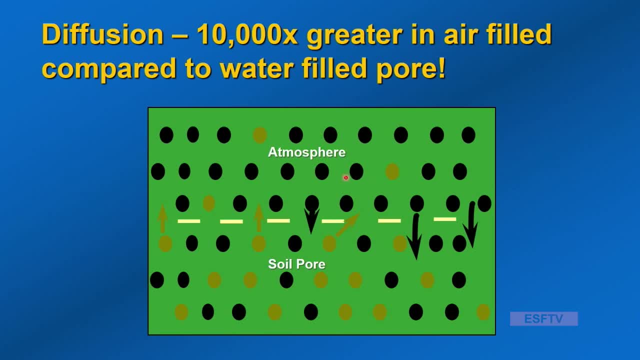 So oxygen, there are a lot more of them- a higher concentration of the atmosphere, 21% to be precise, compared to the soil air. So there's a gradient of high concentration to low concentration of oxygen And that gradient is in the direction. 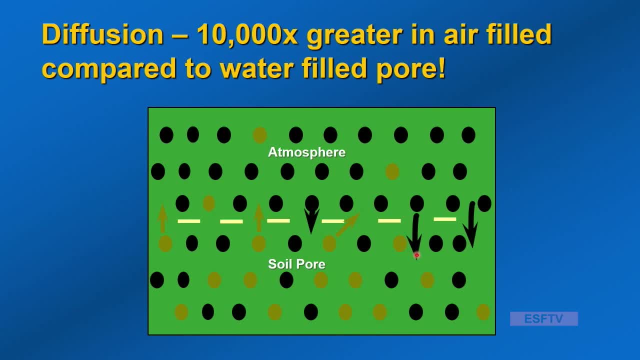 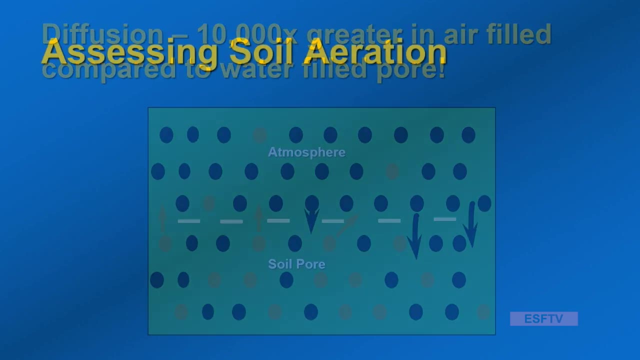 it moves from high, from the atmosphere, into the soil atmosphere. So this is diffusion of oxygen. For carbon dioxide it's the reverse. The concentrations, the relative concentrations, in the soil are higher than in the air, So there's a diffusion. 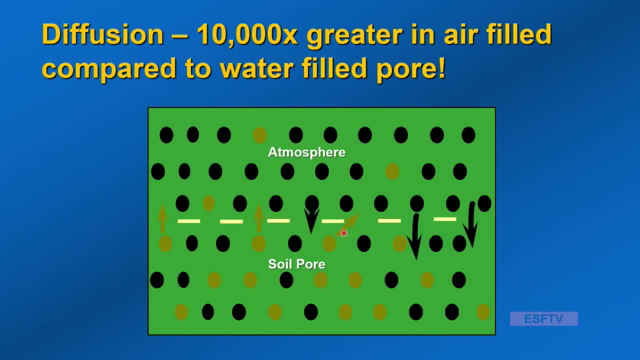 so there's a tendency for those to diffuse out, And so this is the mechanism: diffusion, the movement of molecules and gases in response to a gradient from high concentration to low concentration. And here's a little note, this is worth remembering. 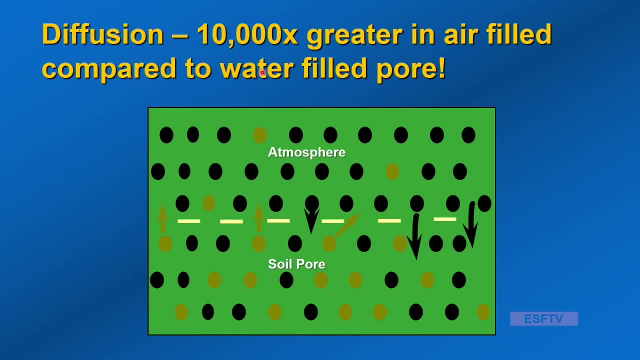 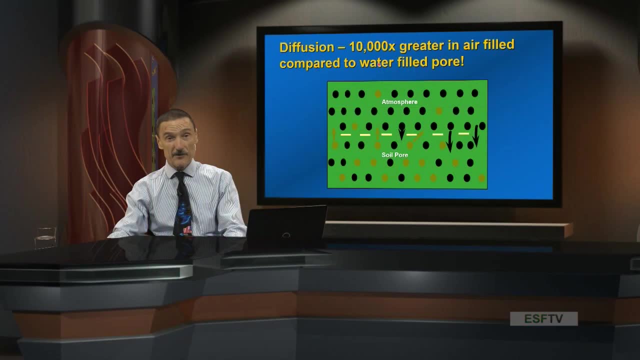 This process. it's 10,000 times greater in terms of a flux, 10,000 times greater in air-filled pore spaces than water-filled pore. So that's saying if you fill a pore with water, you're not going to transfer gases by diffusion. 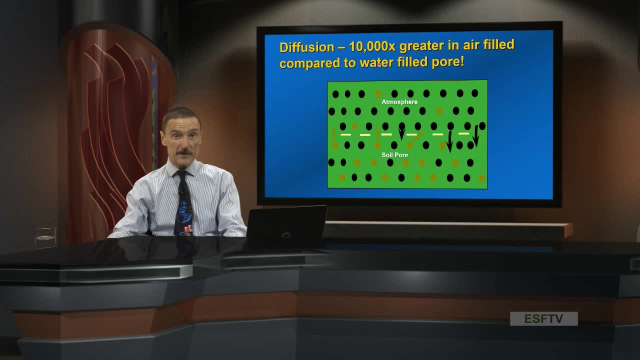 You need a large pore. you've got to have an empty pore, essentially a macropore, or a pore that has no water in it, And then, when you can diffuse, the process will take place. So eliminate those macropores and really eliminate the flux of oxygen. 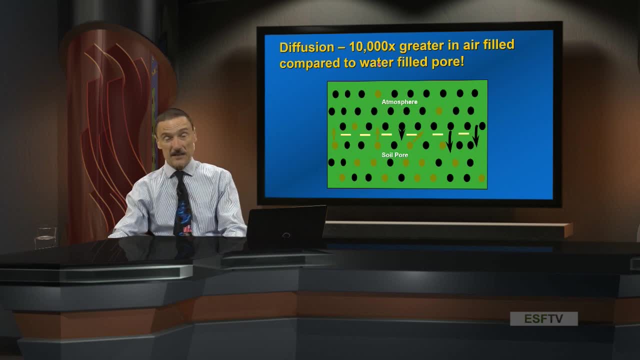 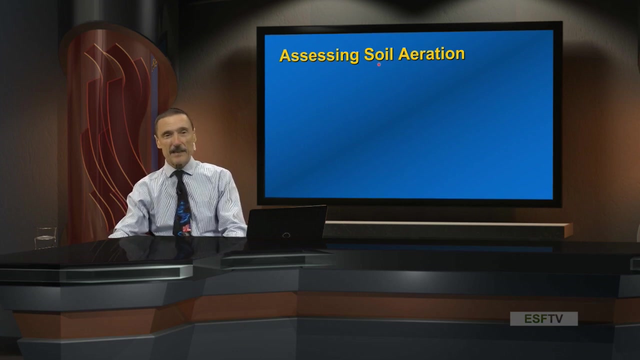 in the flux of CO2 out And limit or constrain aeration. So we've defined it. we think about the process, how it works, and now, how do we measure it? how do we assess it, quantify it? So, in a number of ways, 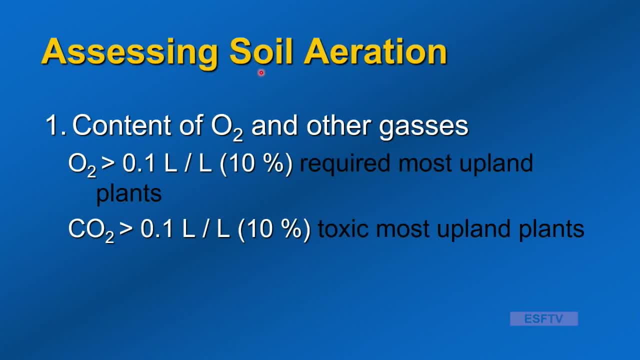 So the first way we can think about it is just the content of O2 and other gases, their partial pressures And so the oxygen. so a general rule of thumb: we need about 10% oxygen to most land plants and most root systems require this. 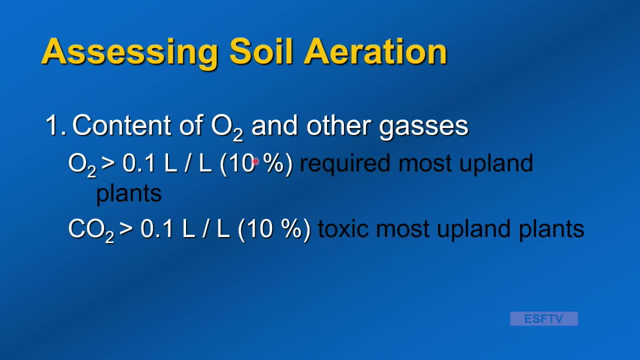 So if you have 10% oxygen in your soil atmosphere, you're good to go. So as you drop below 10%- that's the number- we tend to think about difficulties and limited aeration. So we can look at that from carbon dioxide. 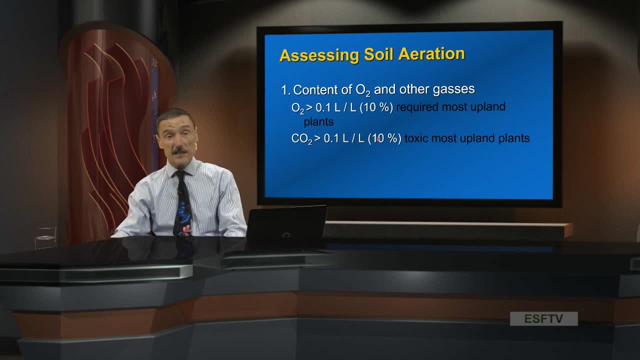 So carbon dioxide, the 10% is the other way. If we exceed 10% concentration of carbon dioxide, then we're in trouble, Right? So either greater than 10% oxygen or less than 10% carbon dioxide, that would be a reasonably well aerated soil. 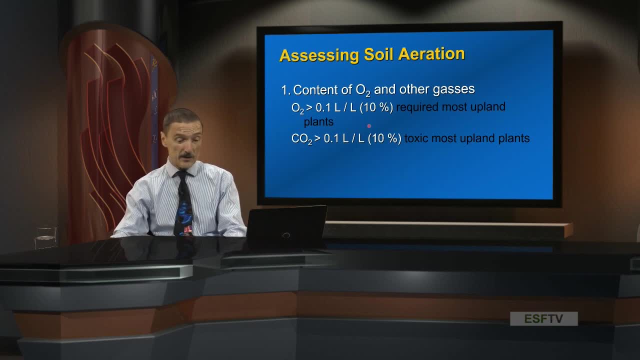 You start to get numbers above and different from those, then that would indicate a poorly aerated soil. So content of oxygen and other gases. first way to do this: When I was a technician at University of Vermont, we used to take samples of 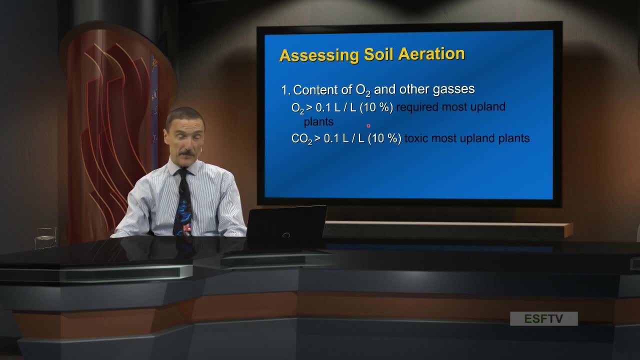 we had looking at soil compaction and we had several of these gadgets, very permeable, actually PVC. we'd cap and we'd cut holes in them so that they would equilibrate the soil air and then we would withdraw gas samples in a syringe. 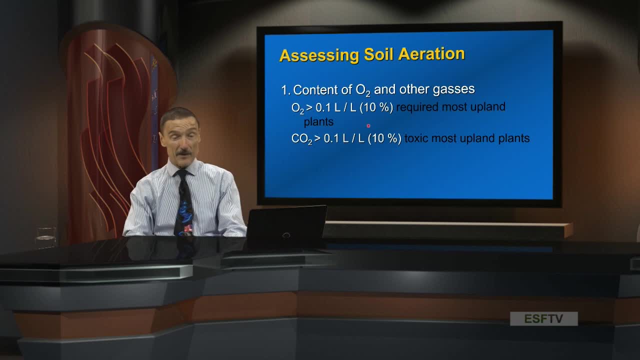 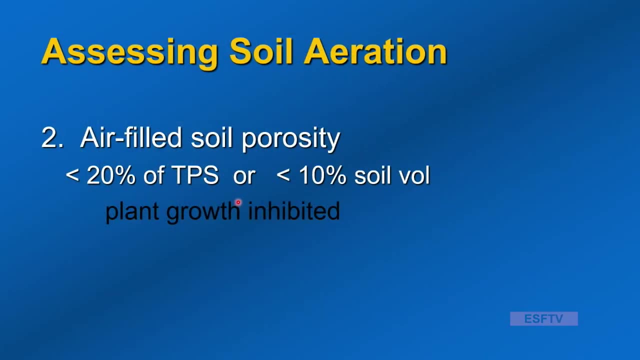 and bring those back to the lab and measure the concentration. So we kind of followed aeration in that way. Okay, there are other ways to do it related. Another way is to think about air-filled soil porosity. Air-filled porosity. 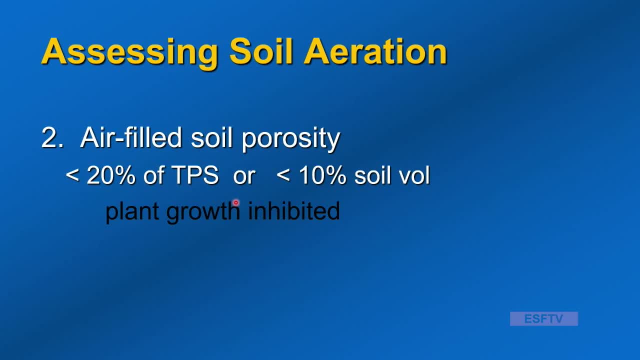 The proportion of soil of the soil pore space filled with oxygen macropores, So generally air-filled porosity is less than 20% of total pore space or less than 10% of the volume that inhibits plant growth. 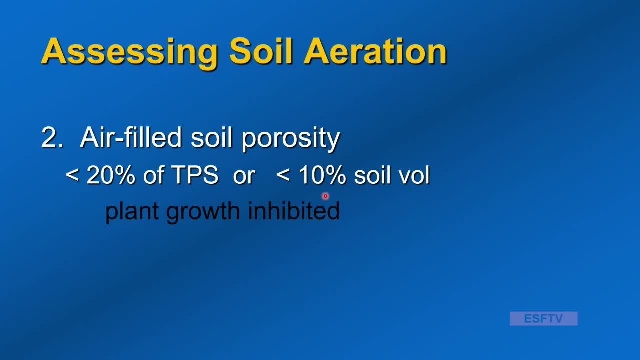 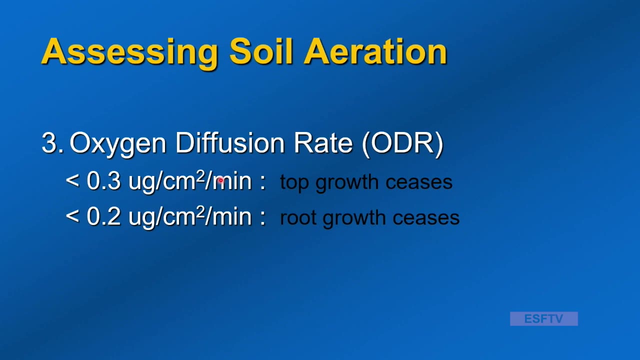 So here's a way to think about a rough idea of aeration, just based on the air-filled pore space. We could get a little more in-depth and a little crazier on the measurement and measure something called the oxygen diffusion rate, abbreviated ODR. 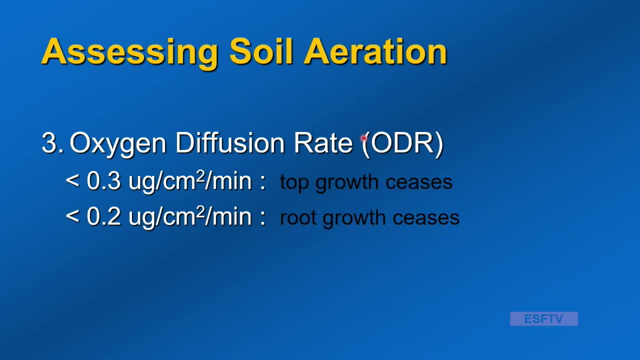 oxygen diffusion rate. And so we measure this. and so this is a flux rate of oxygen and we measure it in the amount per unit area, per time, micrograms per centimeter squared per minute. And here are the cut-off values: They're around 0.3 to 0.4,. 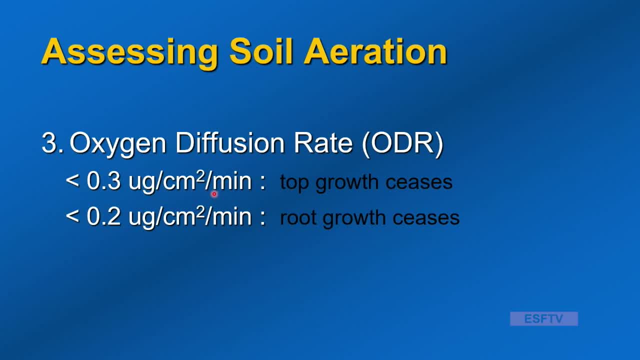 0.2 micrograms per centimeter squared per minute. So below those values we start to see a reduction in top growth and below the 0.2, a reduction in root growth. So this is a threshold measure. 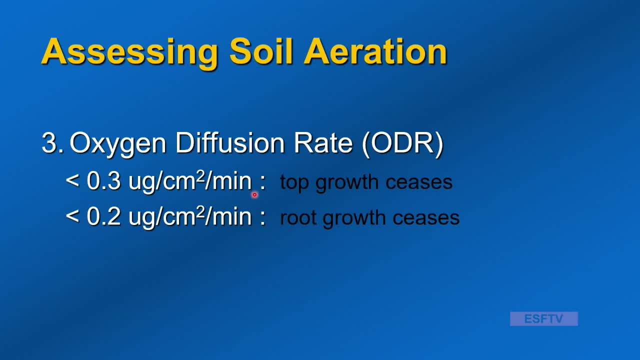 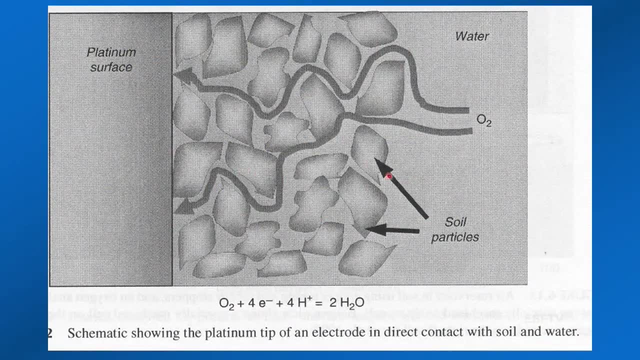 a measure we can put in, and I'll show you a picture of this- We put in a little probe and measure the oxygen diffusion rate. So we do this by these platinum surfaces. Here's an illustration of it. Here's water and soil particles. 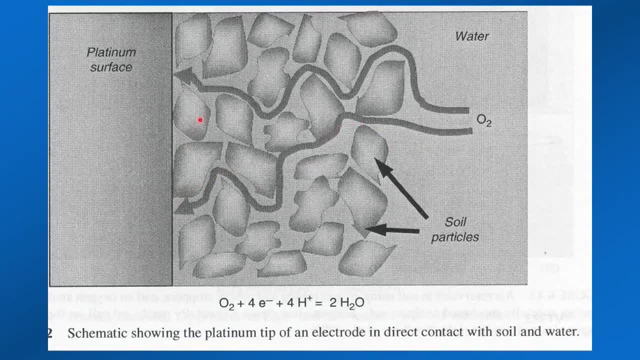 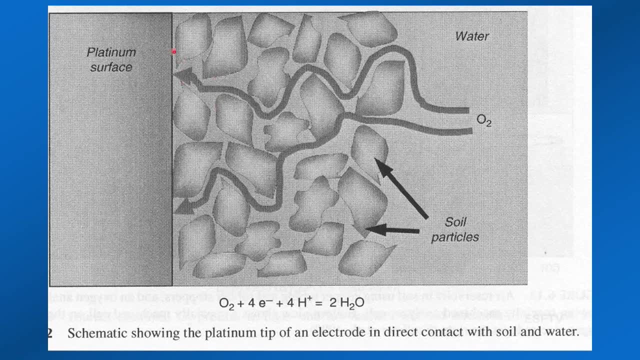 And here's oxygen diffusing to this plate, to this platinum surface, And we can actually measure that, And so we can get a readout based on the difference in electrical potential and essentially measure this rate: micrograms per centimeter squared per minute. 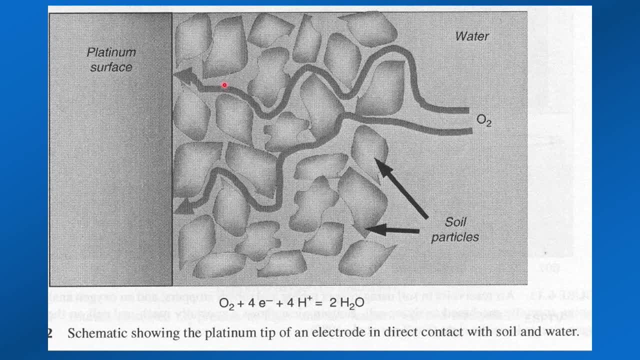 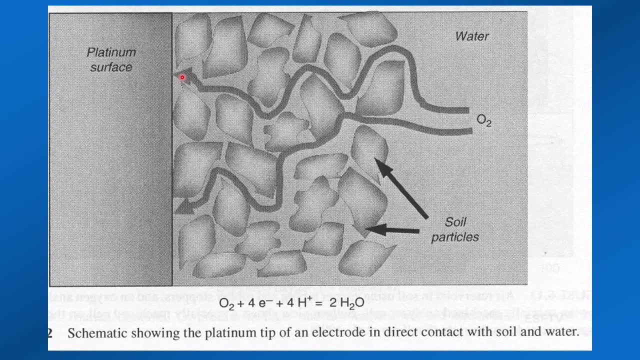 Okay, It's sensitive, It's a tough thing to measure, It's sensitive to how you put in your probe and it's a lot of work, But it's one way to assess aeration that 0.2 to 0.3 micrograms. 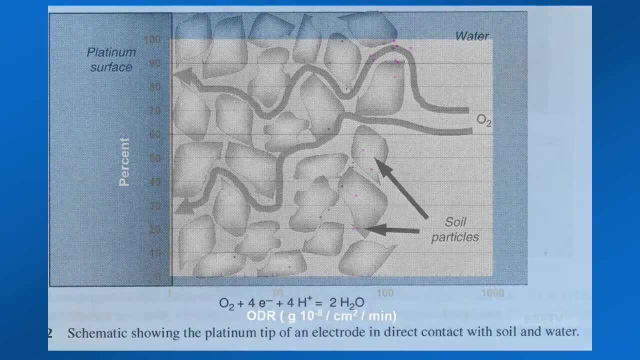 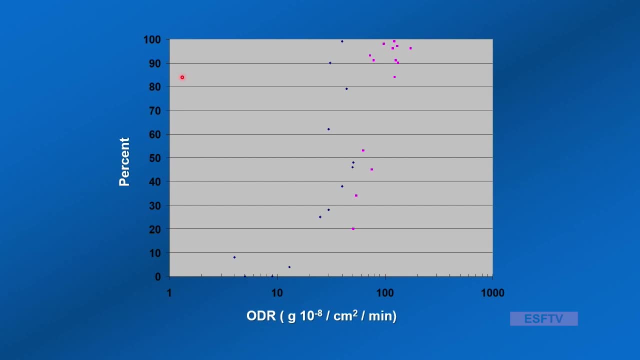 per centimeter squared per minute. So here I've got an illustration of an application of this. So I had a very good friend in Georgia, a colleague. he had a couple of grad students working on this and looking at two things. 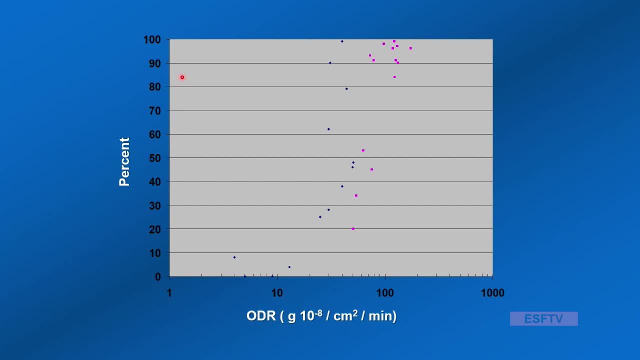 looking at- One was looking at labile pine and one was looking at cotton and some interesting greenhouse studies. And this is They had measured. So Scotty Toriano had measured oxygen diffusion rate And this is 30 units of grams. 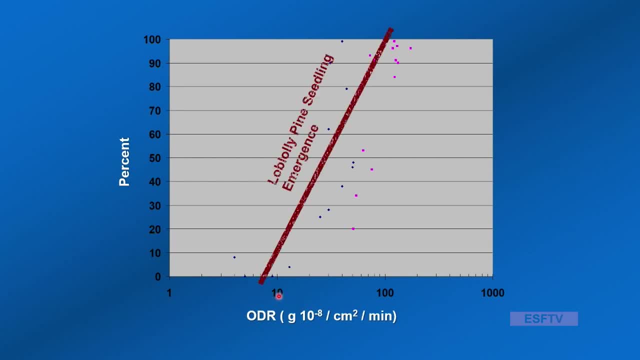 10 to the minus 8 centimeters squared per minute. Okay, And labile pine? So they looked at labile pine seedling emergence and it turns out that the rates increased linearly with the log of the oxygen diffusion rate. 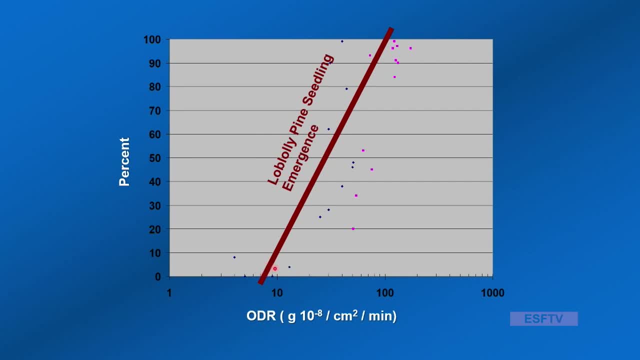 So here we are down at this low 0.2 to 0.3, and then it takes off. So this is an indication of the impacts of oxygen diffusion rate measured directly, based on evaluating the emergence of labile pine seedlings. 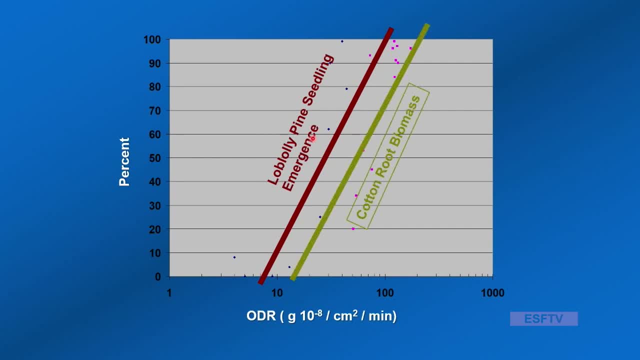 So one biological way to do it, Interesting cotton root biomass. in another study by another grad student, the same kind of rate of change with the oxygen diffusion rate. A linear increase in the percent of cotton root biomass growth as a function of the oxygen diffusion rate. 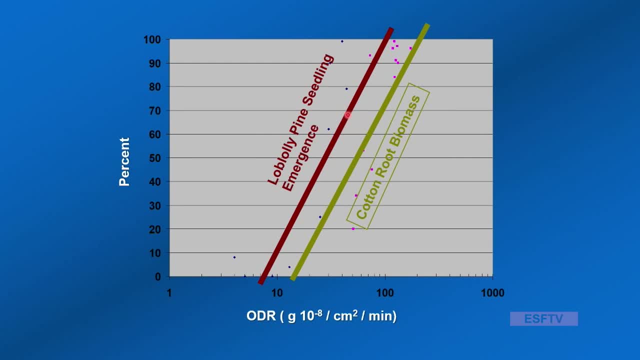 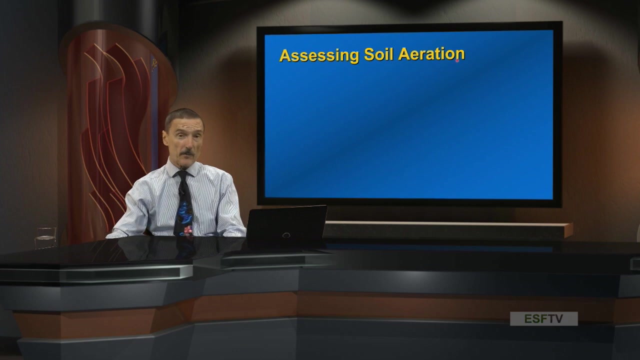 Interesting that they both had the same slope, So kind of neat. Just some supporting data to show these details of these generalizations, Some supporting data. So that's two or three ways and there are more ways to assess aeration. 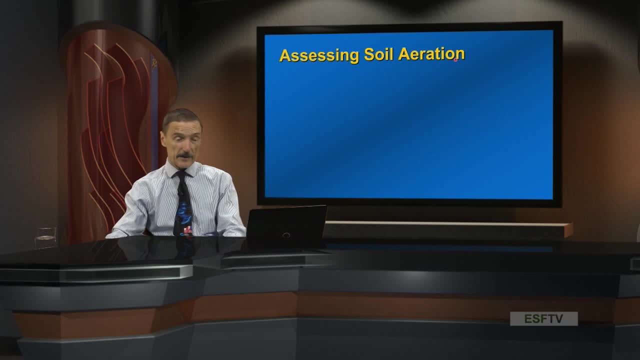 So we've looked at the airfield porosity, we've looked at the oxygen diffusion rate, we've looked at the partial pressure, the concentration of oxygen and CO2.. We had three so far, And let's go on to a fourth. 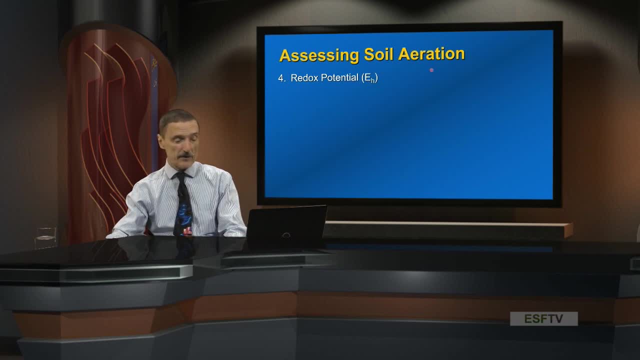 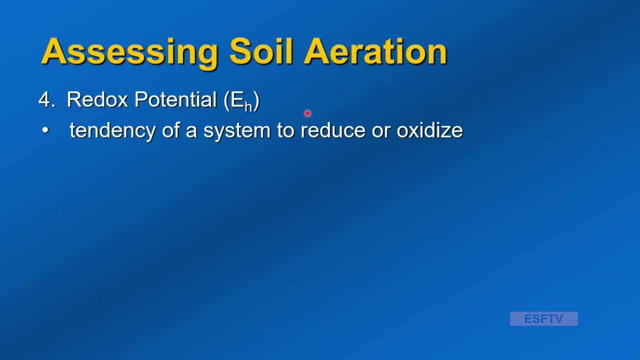 The redox potential. Redox potential, It's a change in voltage. We represent it as Eh, capital, E, small h. So this is a measure, this change in voltage, a measure of a system tendency to reduce gain electrons. 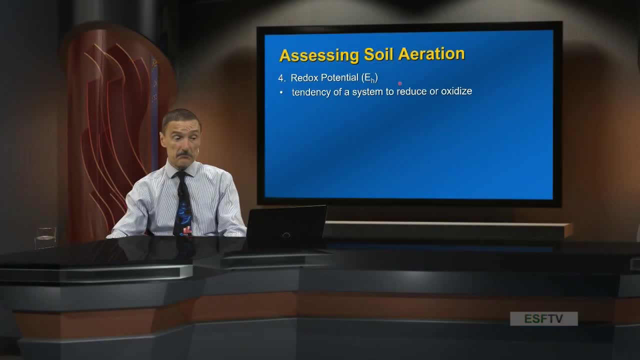 or oxidize, lose electrons, Redox potential, A number, a change in voltage that shows us the tendency of a system to gain electrons or lose electrons, to reduce or oxidize. And so why does this happen? So in our aerobic systems, 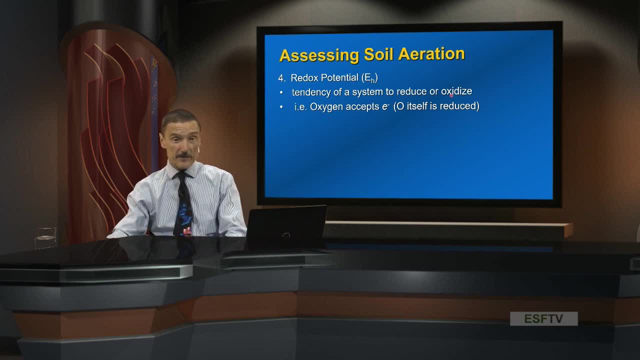 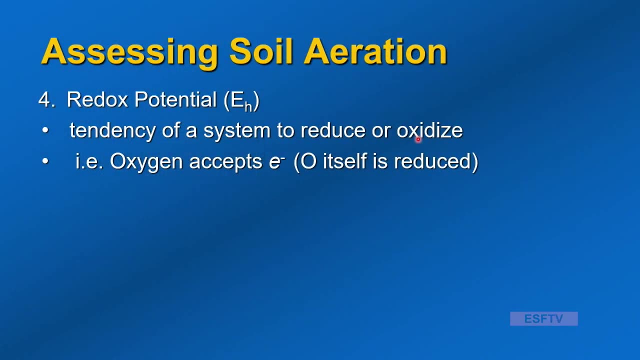 of course we have oxygen around. Oxygen is the electron acceptor, It's driving respiration, it's collecting electrons. Of course, when you oxidize oxygen, when you oxidize something, electrons flow to oxygen. oxygen itself is reduced. 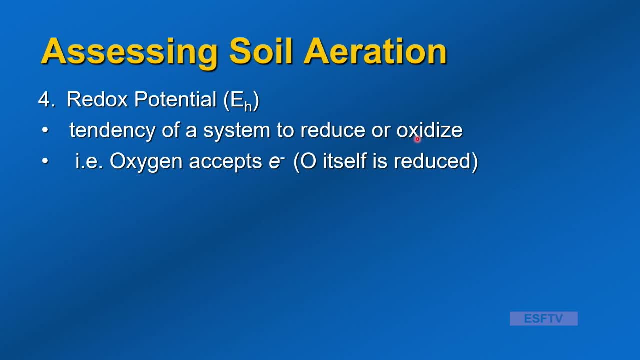 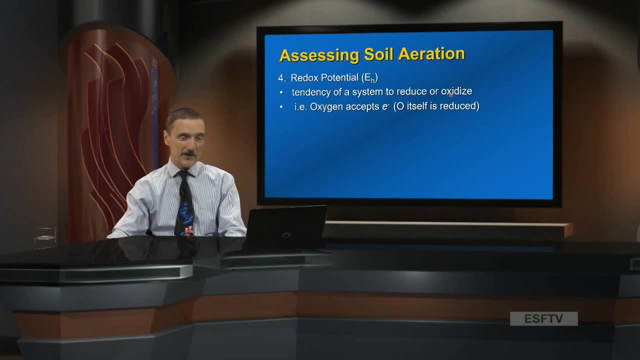 But in aerobic systems, oxygen is taking on the electrons And everybody's happy. plants and animals are going crazy, producing a lot of biomass, respiration's going, the system's happy, and we go on and on. We danced on and on. 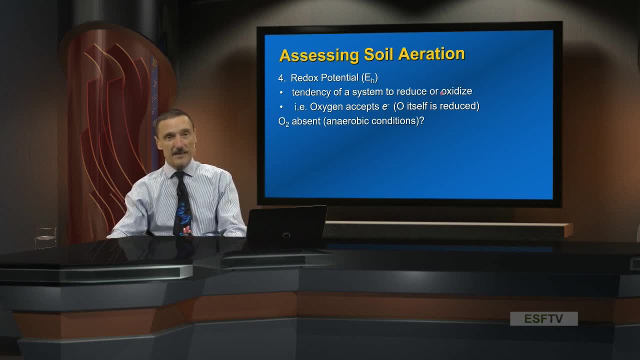 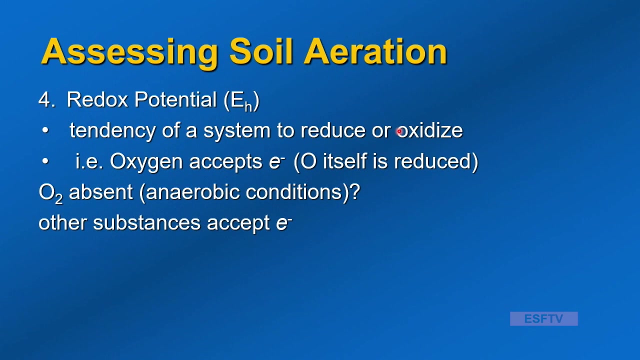 Now what happens, though, when you run out of oxygen? And so that we understand that as becoming anaerobic, a lack of oxygen, anaerobic systems, And this has an impact, and we can measure it, and we think about assessing soil aeration. 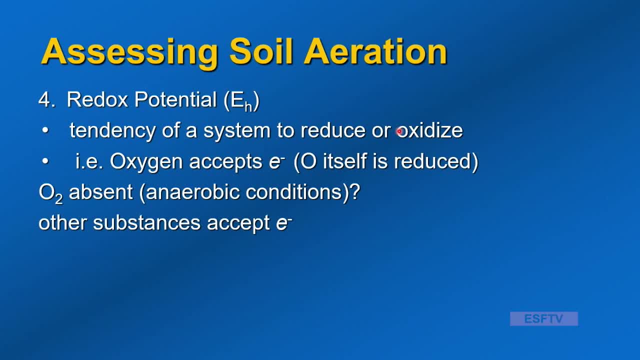 So what happens when oxygen becomes scarce or is no longer around to take or accept the electrons? Other substances accept the electrons, Oxygen is open for business, oxygen closes for business and the system goes on, albeit much slower, right. Aerobic systems are extremely efficient. 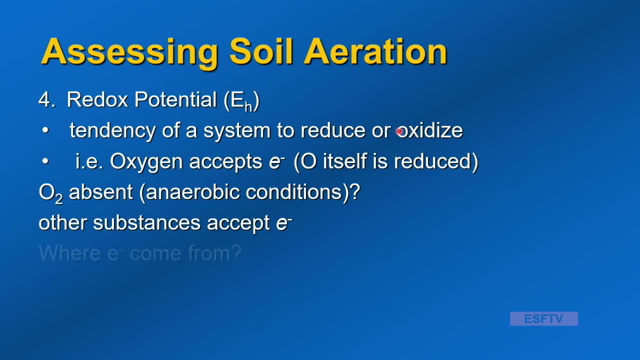 anaerobic systems a fraction of the efficiency. Where are all those electrons coming from? Respiration- Respiration- The organism's breaking down sugars trying to make energy. Respiration- What's that look like? That's glucose. Glucose- is that six-carbon sugar? 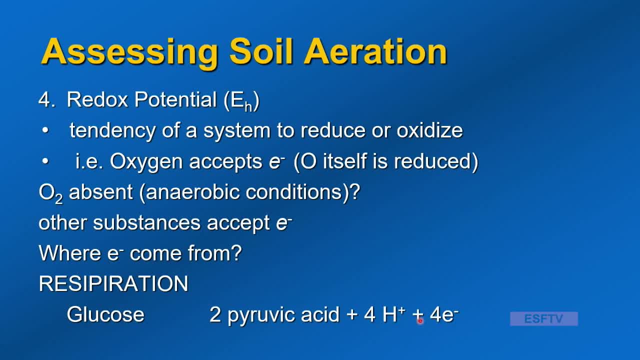 It's converted to pyruvic acid, hydrogens and electrons- right, So this is a part of respiration: Glucose converting to pyruvic acid. If you take biochem, you go through this whole thing. you go through all these cycles. 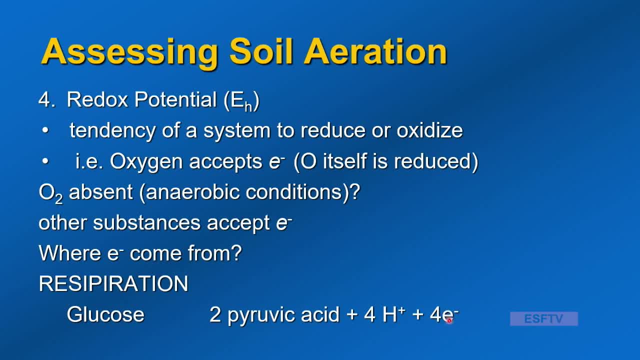 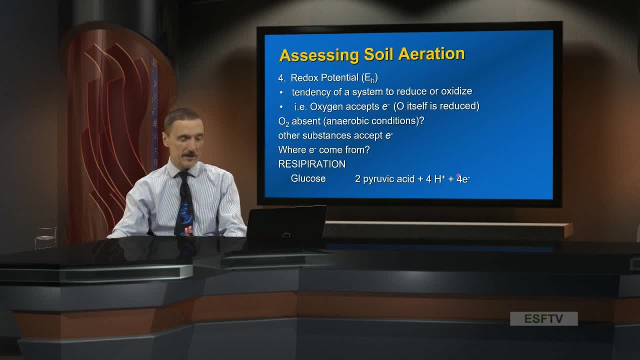 but for now, this just is an illustration showing you that respiration generates electrons. That's the bottom line here: Respiration generates electrons. Glucose, of course, is the sugar that runs a lot of our processes. We burn up sugar. 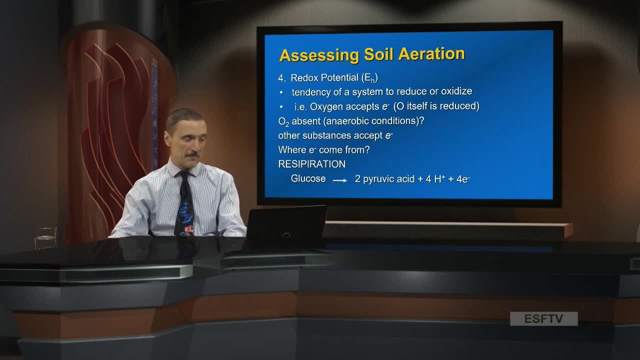 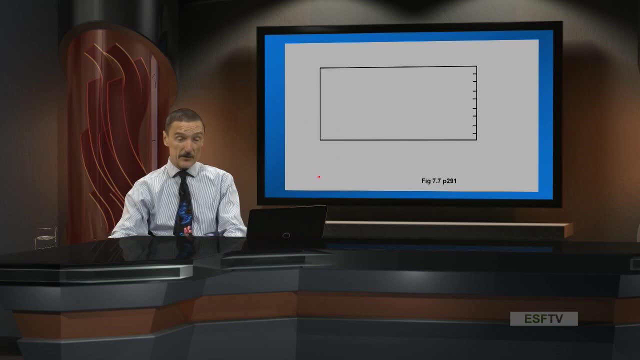 we get energy. throw a little bit on my ice cream. So eventually, if you don't put the oxygen in, it doesn't keep aerating, you don't move through, you run out. And let's look at what happens over time. 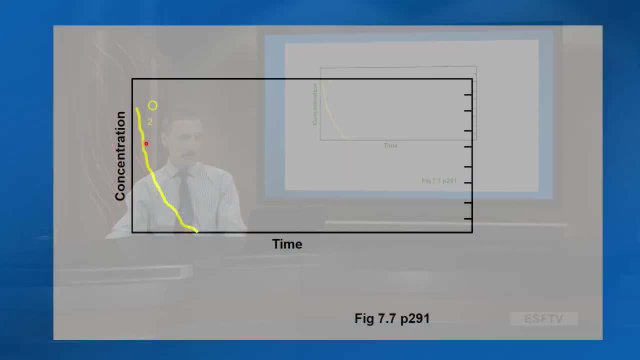 So here we have. we don't put the oxygen back, it takes a nosedive. So this is out of the text. this is figure 7-7 on page 291.. So here we are, depleting oxygen, not aerating. 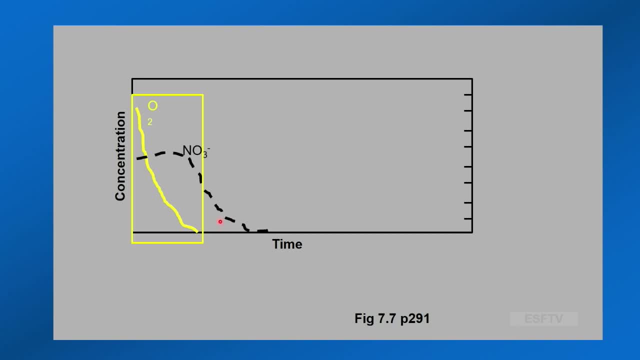 and it's going down, down, down. At the same time, nitrate is around, so nitrate is the next one down the line. so when oxygen gets low, nitrate becomes the electron acceptor. It's the next one on the. 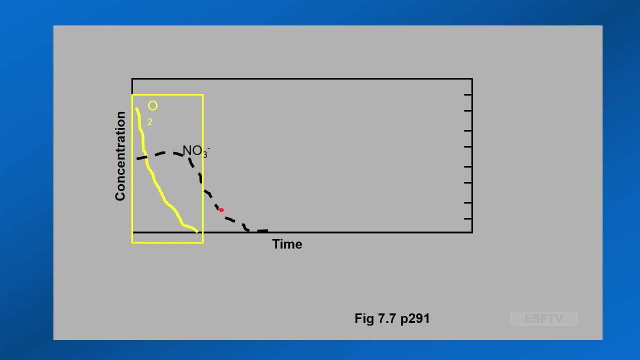 electronegative species that will take on electrons. So this is an illustration of what's going on with this EH measurement. We're going from 6.72 to 6.52 to 5.2.. The EH is dropping. EH is dropping. 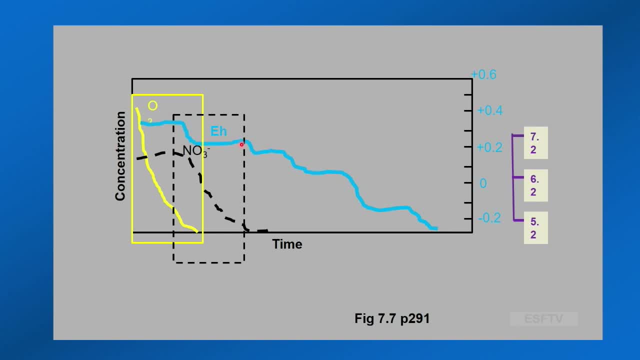 You can see that as we run out of oxygen and eventually we run out of nitrate, EH is dropping further. What's happening then? Manganese starts to pick up the electrons. Manganese is reduced, It takes the electrons, EH drops. 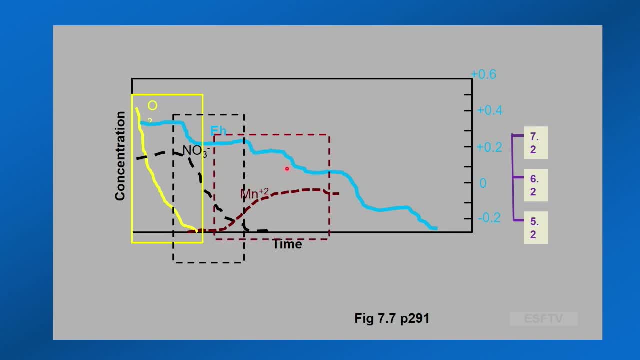 EH drops further. Iron, You know our old friend iron, becomes reduced. EH drops further. It's picking up the electrons, Hydrogen sulfide. We run out of iron, Hydrogen sulfide becomes the main collector of electrons, that stinky swamp gas. 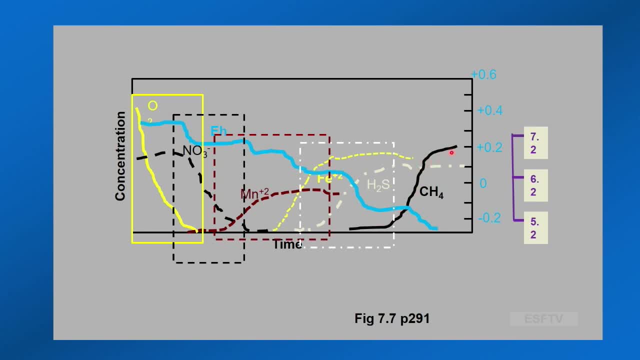 And then, last, we really reduce conditions: Methane, We produce methane. What's happening to pH? The pH is going up in this system as they become more and more anaerobic. So, as they become anaerobic, wetter and wetter. 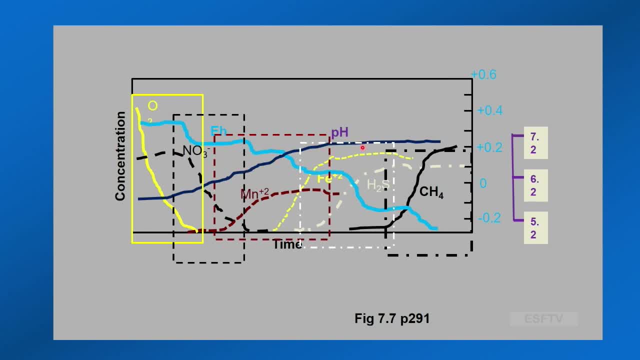 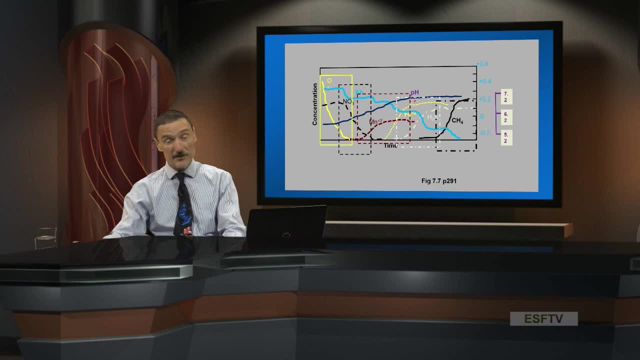 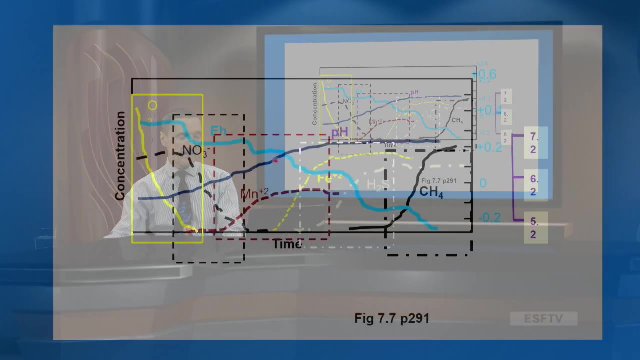 less and less dissolved oxygen, less and less dissolved everything going down the tubes, so to speak, the anaerobic tubes. that's interesting. We'll talk a lot about pH in our last unit, our last lab, but for now just note. 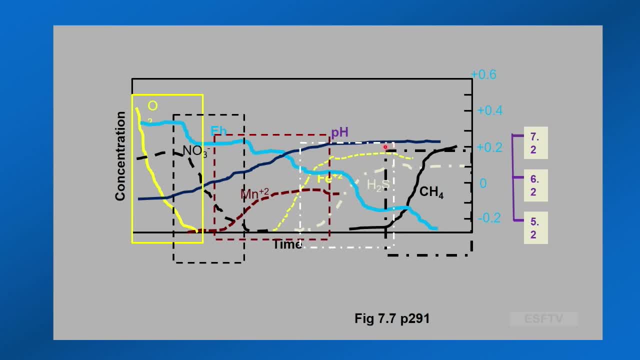 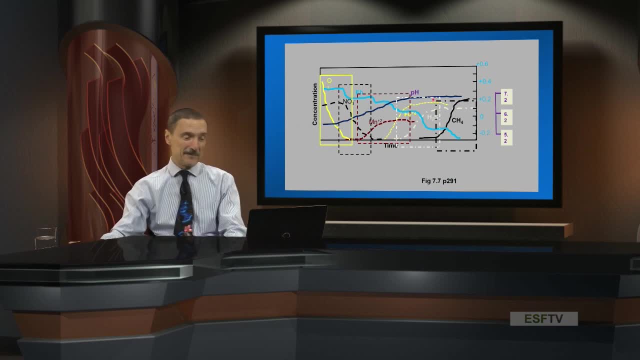 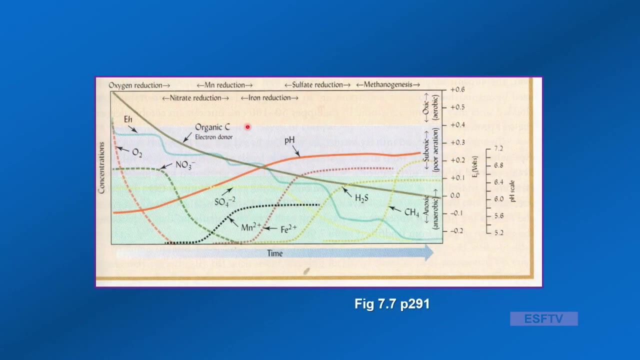 that as we become more anaerobic, the drainage becomes poorer. the pH tends to go up. We'll explore that later, Not much later. a few more weeks, the semester will be over. oh my god. but one thing at a time. 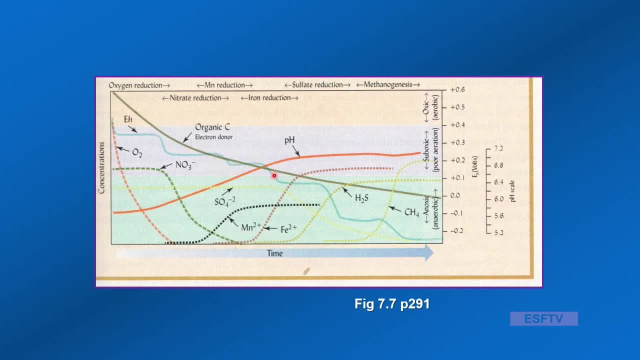 In the text. pH going down. this is the same pattern, but now with some nice colors. pH going up: oxygen depleted nitrate picking up the electrons. nitrate depleted sulfate picking up the electrons, manganese, all the way down to. 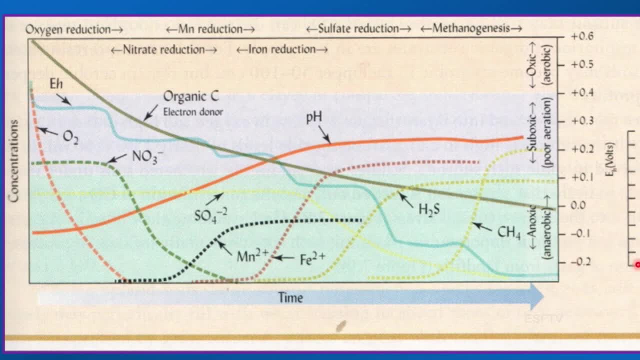 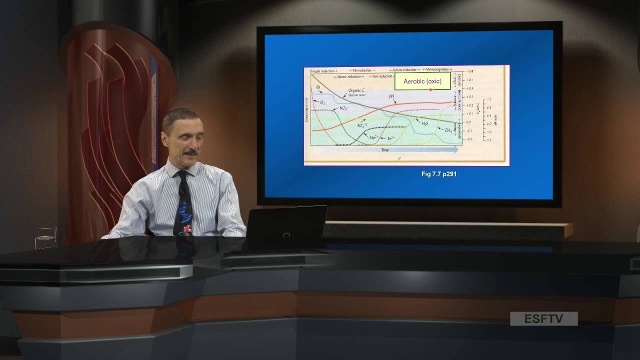 production of methane, Showing the pH dropping. here we are at 0.6, dropping down to minus 0.2. along with these processes, Aerobic up here, aerobic oxygen, around oxygen disappears. what do we call this? 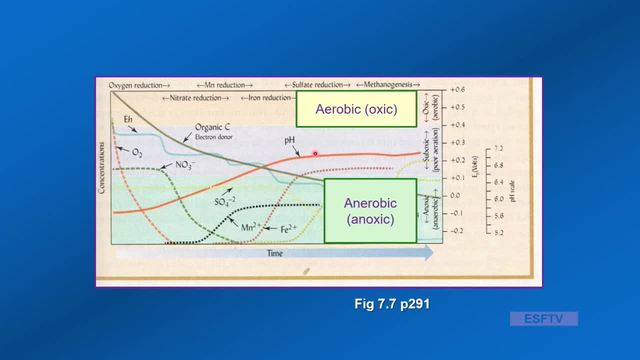 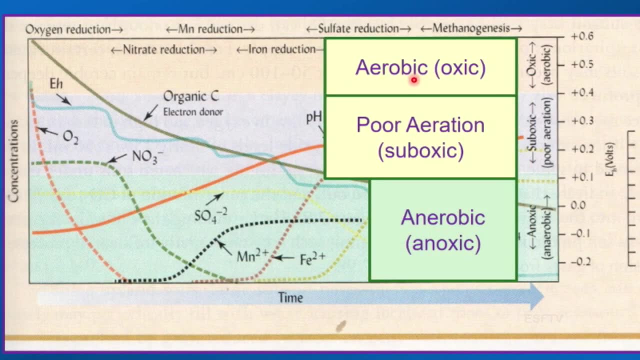 Anaerobic, so we get below down here and we're anaerobic. Poor aeration, so we go from good aeration to poor aeration to anoxic. oxygen depletes, other electron acceptors pick up the electrons and we produce stinky hydrogen sulfide. 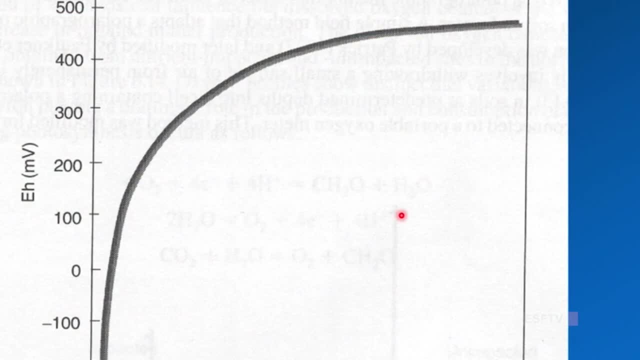 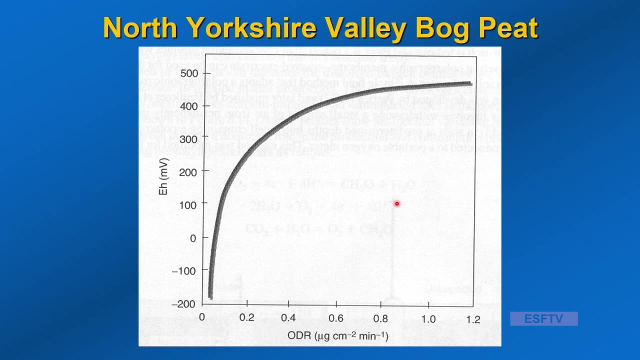 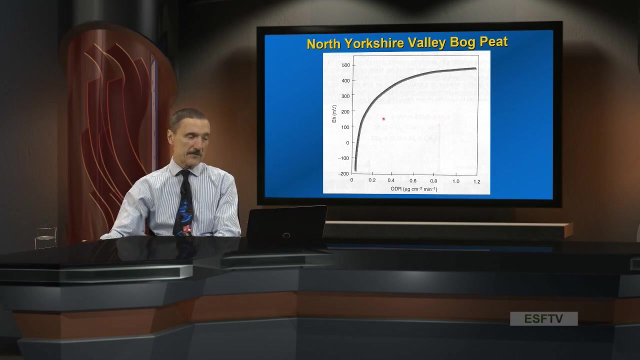 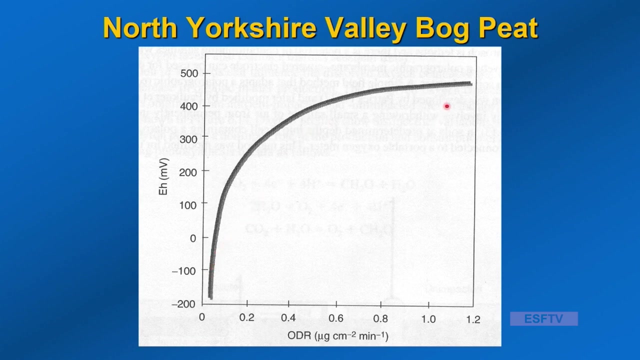 when we get down here. So we could think about that. we've thought about that as EH and now we can think about that in terms of oxygen diffusion rate and these are some data from the Valley Bog peat showing the pH and how that relates to ODR. 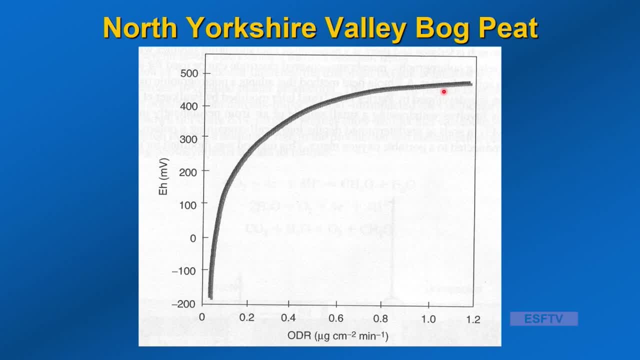 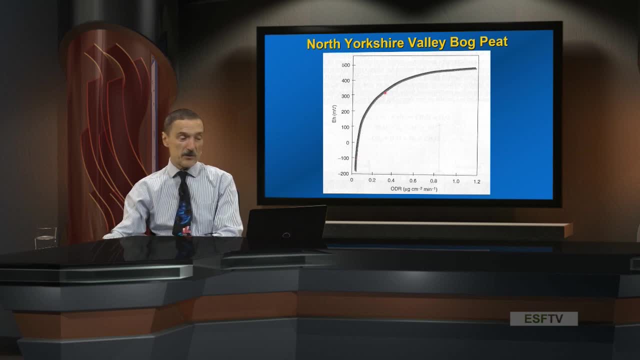 So you might expect, since these assess aeration and anoxic conditions, that they're related, and indeed they are. So as the ODR increases- remember that's one measure. we have down here the 0.2 to 0.3 micrograms. 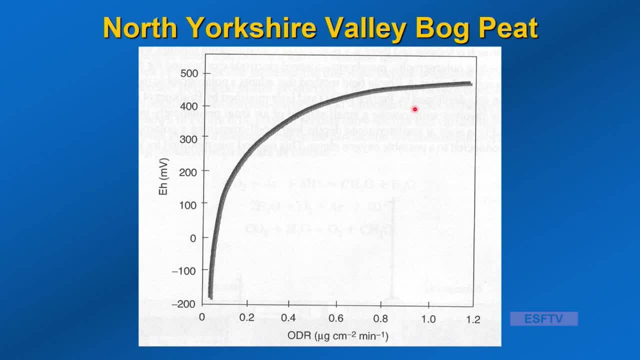 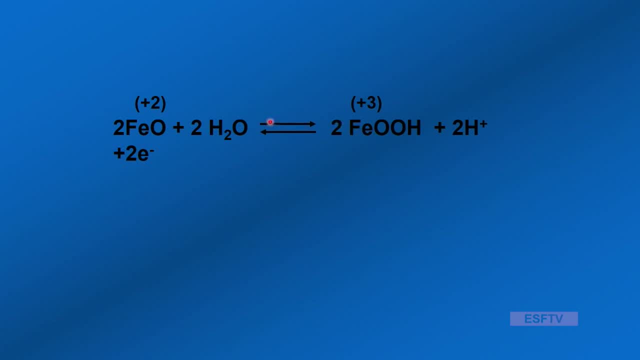 per centimeter squared per second. as that increases, the EH increases. so they are related. So how about those electrons? So here's a picture of FeO plus 2,, FeOH plus 3, and this is where FeO accepts electrons. 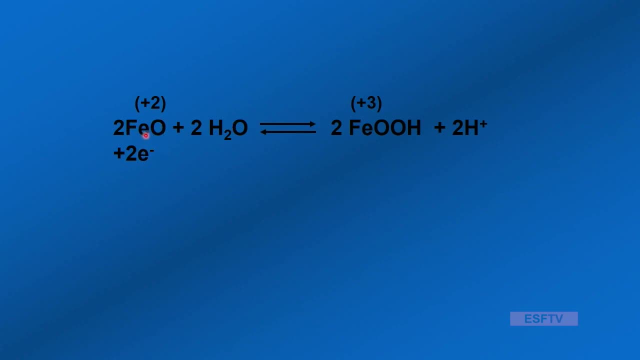 and electrons do it, make it to FeO plus 3. Irons oxidize. where do the electrons go? The electrons go to water, And to do that we have to make sure that the electrons are in the water. You've got to have oxygen. 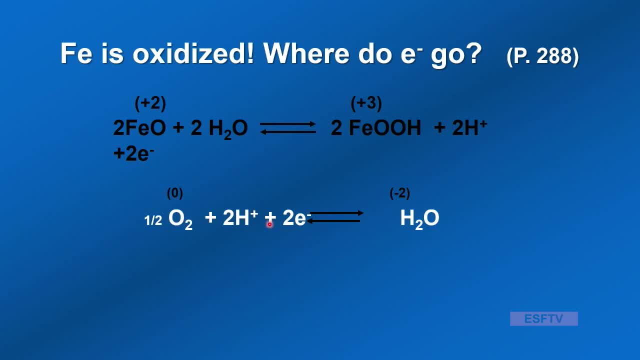 So thankfully, oxygen is around. it accepts the electrons. What happens when oxygen gets electrons? It's reduced to water. No problem, as long as you keep feeding the oxygen in. The electrons go to O2, what must be reduced- Oxygen is reduced. 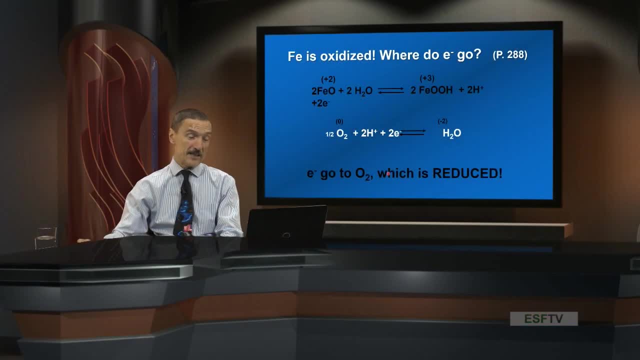 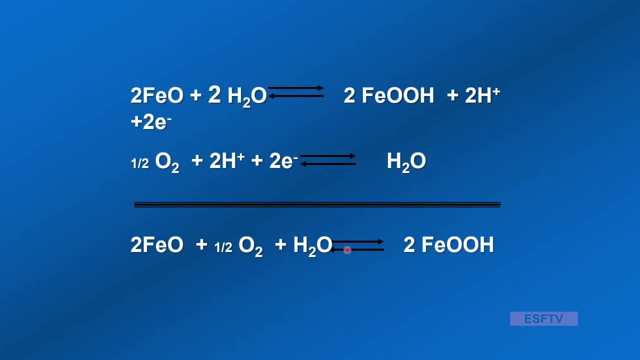 But it's doing the oxidizing Cool right. And so when you see this little system of FeO to FeOOH, going from oxidized to reduced, this is the thing you see, But what we always leave out is all the little details. 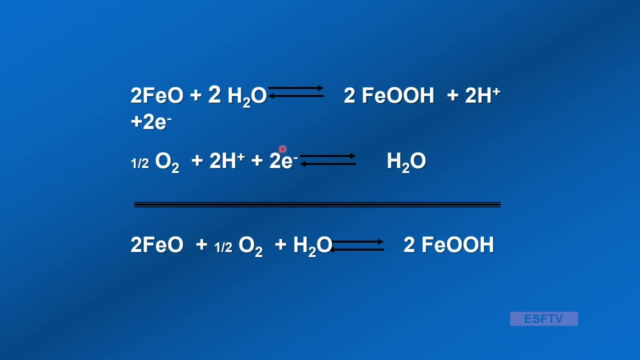 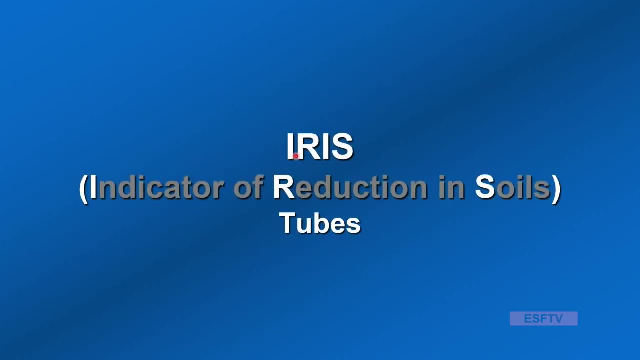 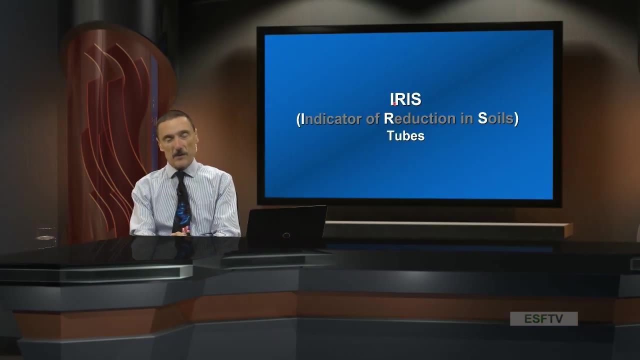 So the little details remind you that the electrons are moving on. You gain electrons and you reduce something, You lose electrons, you oxidize something. So those are some quantitative ways. There's still other ways. It's kind of quantitative, I guess you'd say quantitative. 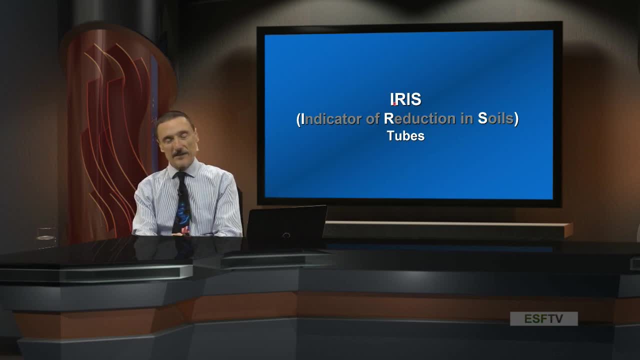 and we'll talk about why. But one of these new methods- this is out in the last 10 years, some work that Marty Ravenhurst and others had done at the University of Delaware, something called IRIS, And IRIS for short. 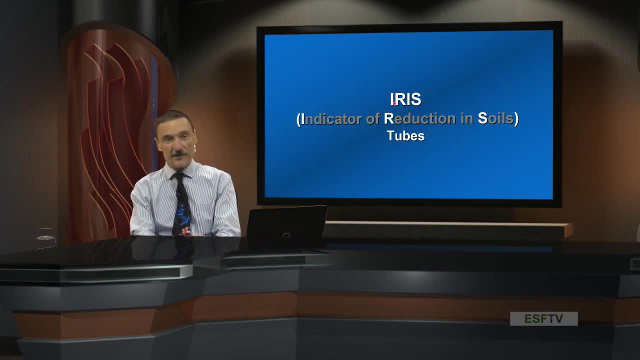 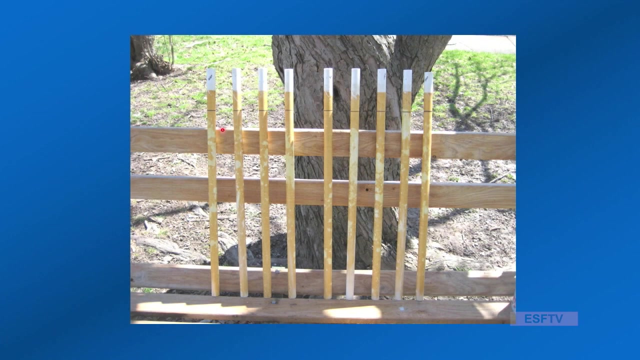 or a demonic for Indicator of Reduction in Soils, IRIS, So kind of neat. So, essentially, you take these tubes and paint them with an iron oxide paint to dissolve them off. Here's a picture of these. These are samples from increasing anoxic conditions. 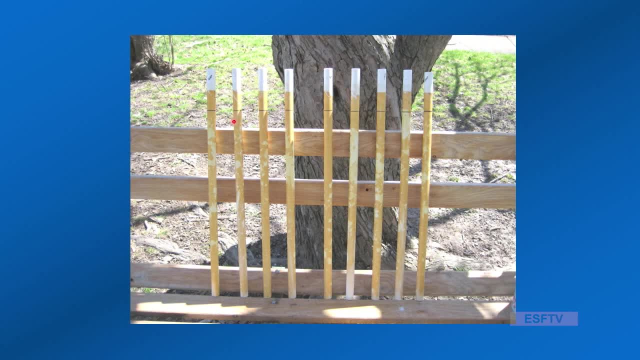 as we go from wetland, And what happens when you put these in the ground. If things are anoxic and you don't have dissolved oxygen, the iron is reduced and the paint peels. So you have a visual expression of the degree of anaerobic conditions. 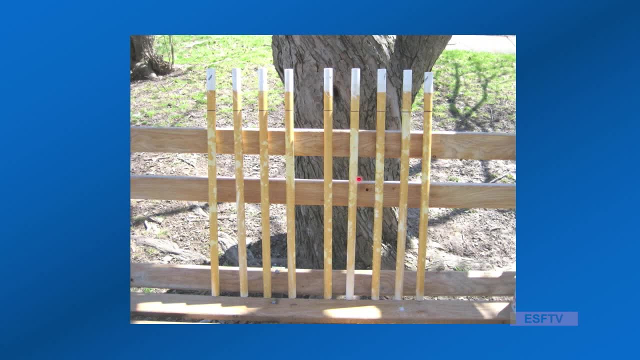 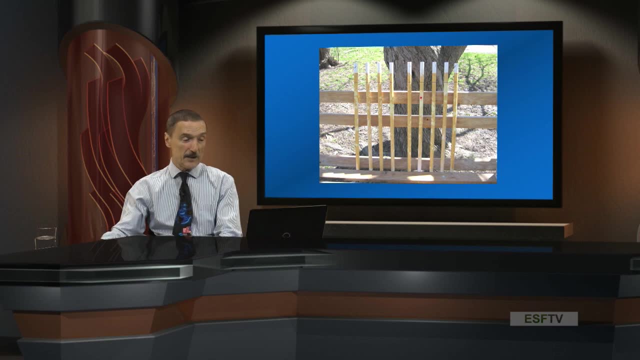 Because iron is being reduced and when it's reduced it's soluble and off goes the paint. So you can actually take these and you can convert these and measure the area using a little bit of photo technology and come up with a quantitative estimate to try to relate that. 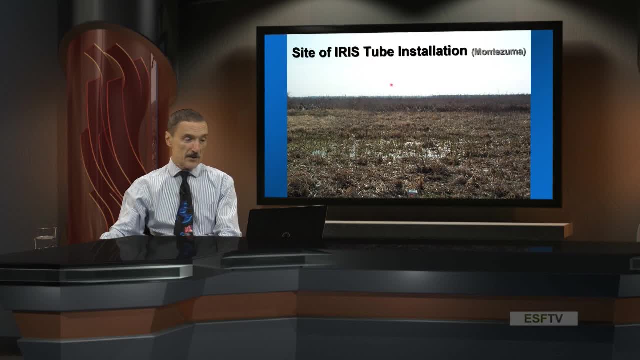 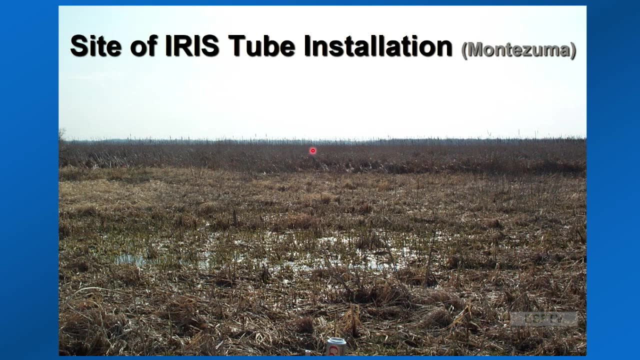 to these other measures. So this is what we had. Those pictures were from a site we had at Montezuma Refuge. This was about 10, 15 years ago now And, to try these out, we were out looking at these And clearly wetlands. 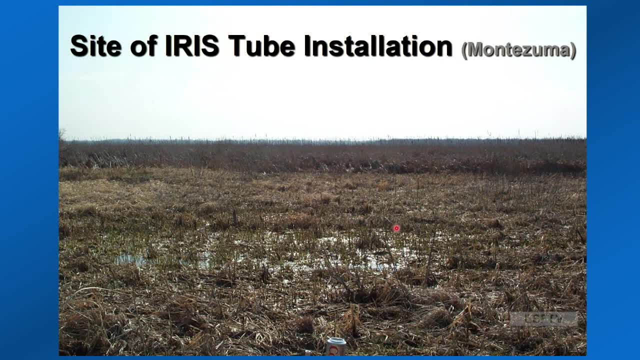 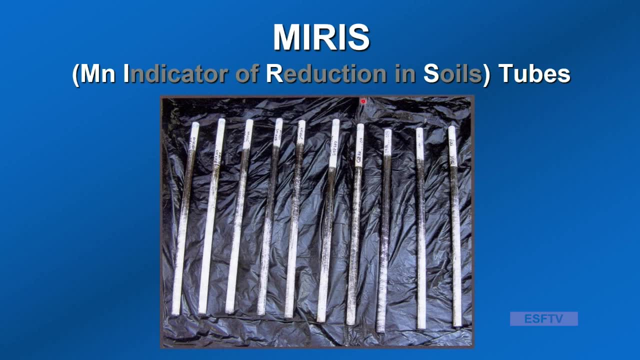 clearly anaerobic, clearly in anoxic conditions, And they performed very well. There's another set of tubes, miris, So manganese indicator of reduction in soils. So iris was iron and these were manganese, And so why bother? 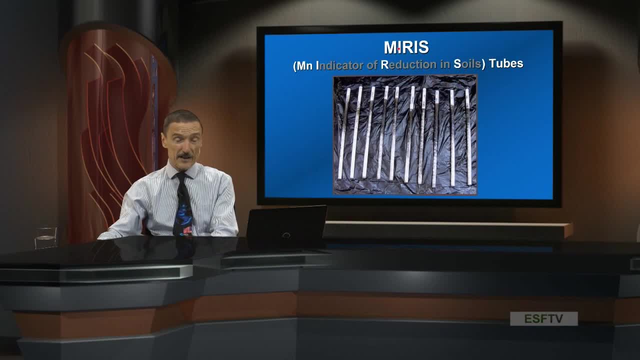 Well, manganese, when you get into higher pHs, sometimes it kind of stops some of these reactions. So when we're into higher pH systems, manganese, manganese, indicator of reduction in the miris tubes And the same deal As you get into more inoxicant conditions. 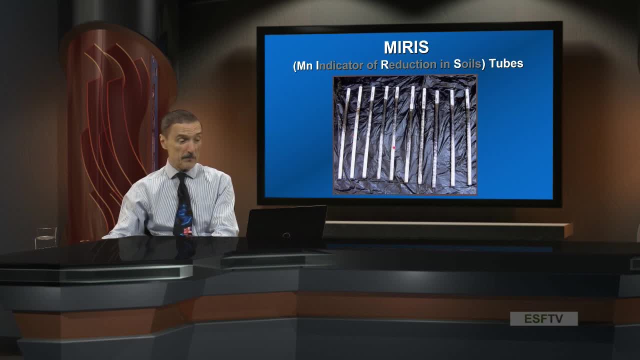 the manganese is reduced, gains electrons, and then this is the result: the paint peels, And this only takes within a month this occurs. So it's kind of a quick and rather relatively quick and easy way to determine aerobic conditions. 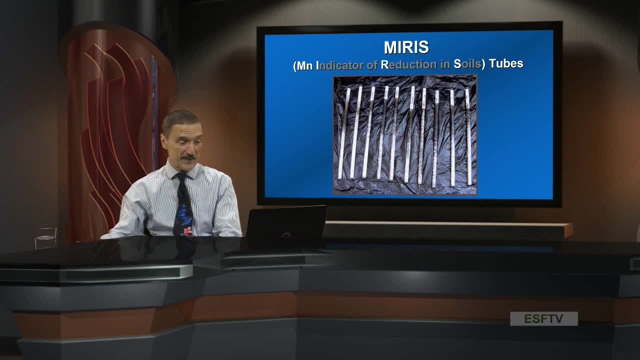 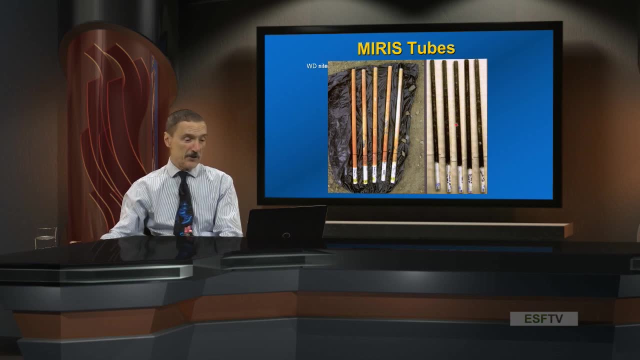 So it's just that, and again relatively recently, the last 15 years. So I think this is pretty cool. So here we have miris tubes all labeled, going down and here in well-drained sites. So let's. 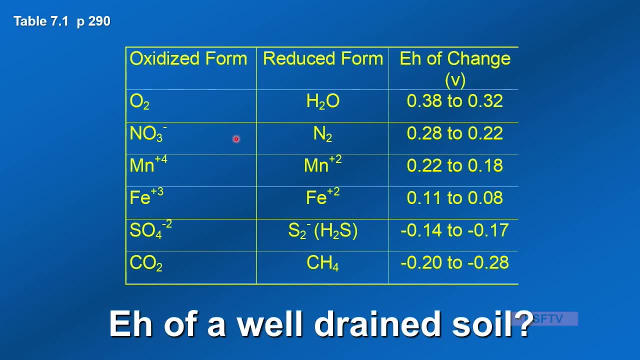 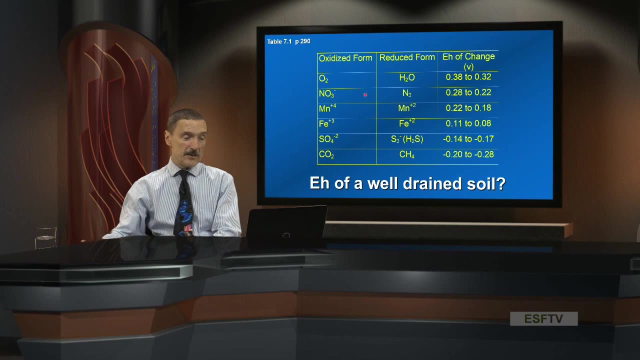 if we can think about. back to EH, what is? and we had quantity, we had a number measured in volts and we might ask what is the EH of a well-drained soil As an indicator of aerobic conditions? And so 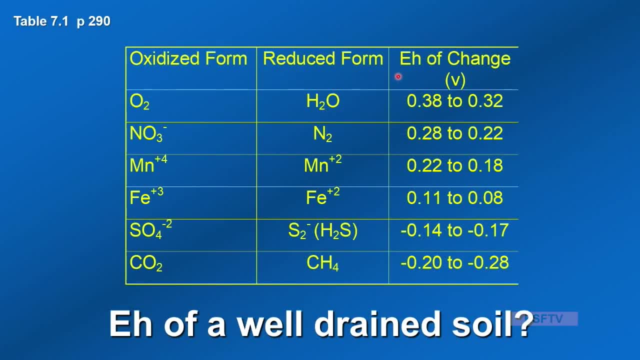 let's look at what happens. Here's the oxidized form and reduced form, and the EH change. So oxygen, O2, it's reduced. when O2 accepts electrons, it's reduced to water And then it's all turned to water. 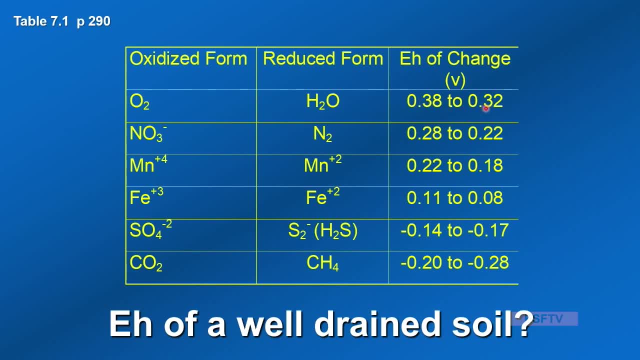 The EH changes so somewhere between 0.38 and 0.32.. So above here this is relatively aerobic. As you go through this phase you're getting into anaerobic, And so next on the list. remember our cartoon. 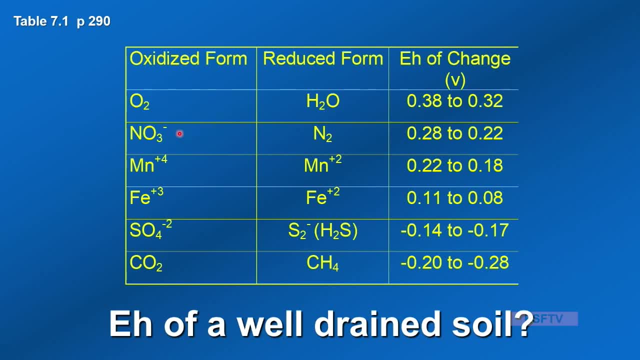 nitrate. nitrate became the electron acceptor. run out of oxygen, nitrate picks up the job. nitrogen gas N2.. And this occurs as this depletes somewhere between 0.28 and 0.22 volts. 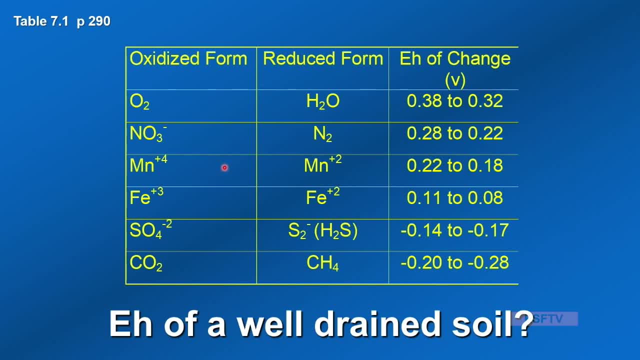 Manganese is next, and this follows right along with the cartoon. we just showed the diagram out of the book. taken apart in my little dots and dashes, Manganese is reduced plus 4 to plus 2.. It takes the electrons. 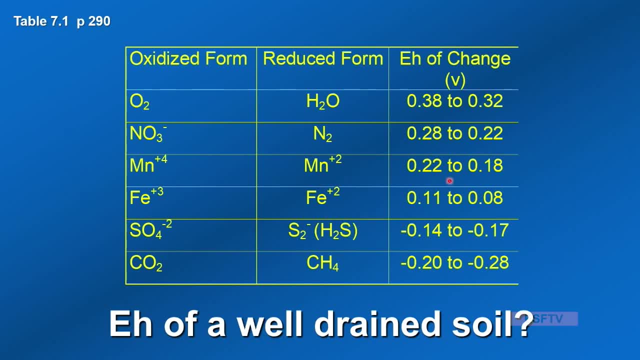 And now we're looking at an EH change. as this becomes depleted, the 0.22 to 0.18 range After manganese, iron, Iron plus 3 is reduced plus 2, it's gaining electrons. and now we're changing. 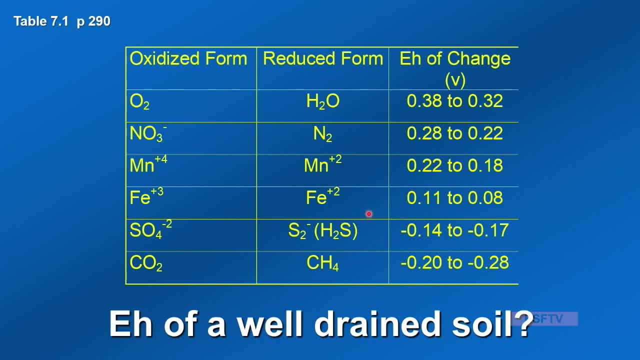 you're going through the EH range of 0.11 to 0.08.. By the time you get down to sulfate, you're producing hydrogen sulfide gas, and now you're down to negative numbers And then finally, carbon dioxide. 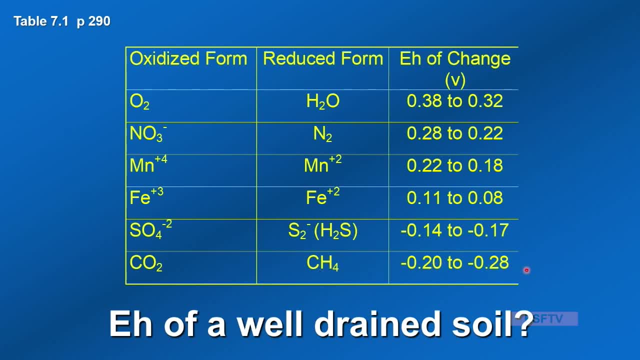 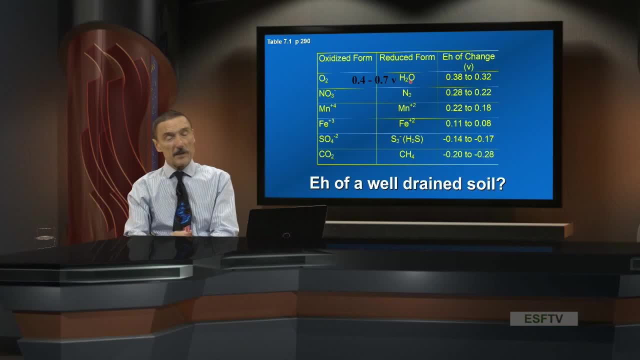 the acceptor to methane very negative numbers. It's toxic and, above here, aerobic. So we could ask, we could look at this and say, what is the EH of a well-drained soil? And if we were to look at this, 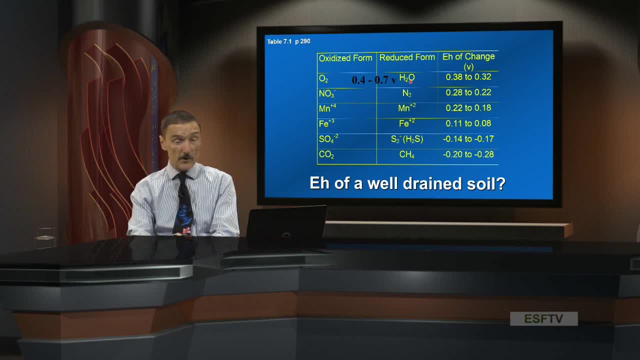 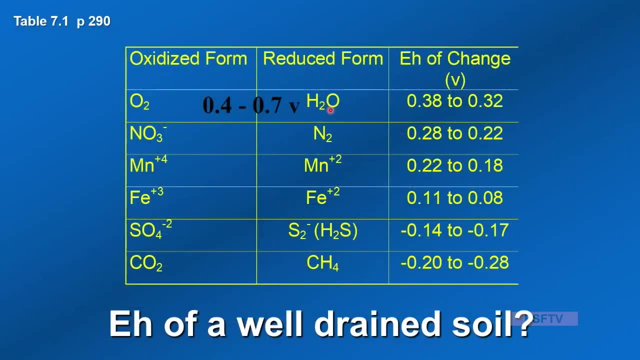 and think about where oxygen is depleted, we'd have to conclude that the EH of a well-drained soil is somewhere between 0.4 and 0.7 volts. So this is a threshold. So we have thresholds so far for oxygen concentration. 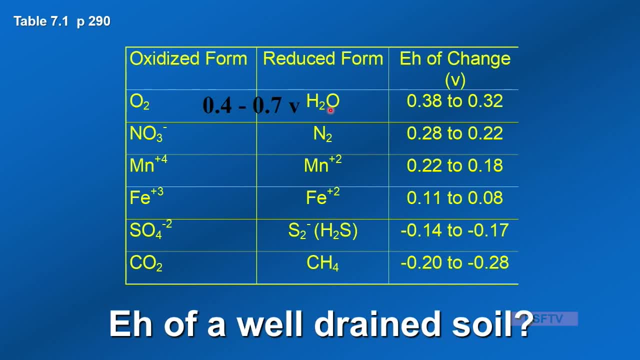 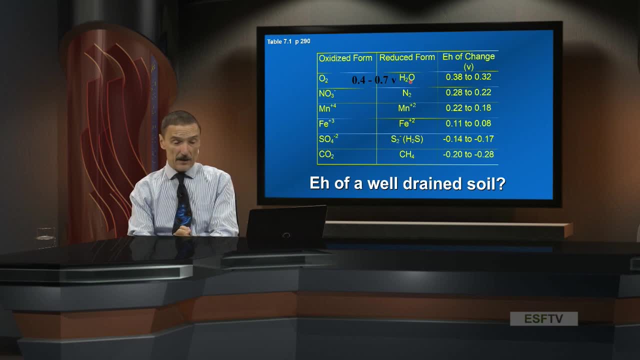 air-filled porosity. we have thresholds for CO2 concentration: 10%. we have thresholds for EH or the. yeah, this EH 0.4 to 0.7 volts. We have a threshold for the oxygen diffusion rate. 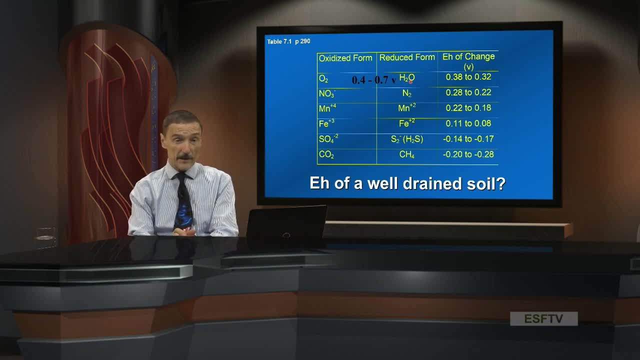 the ODR 0.2 to 0.3 micrograms per centimeter cubed per minute centimeter squared. So we have a number of different thresholds that we can use as little tests or little indicators of do. we have a well-drained system? 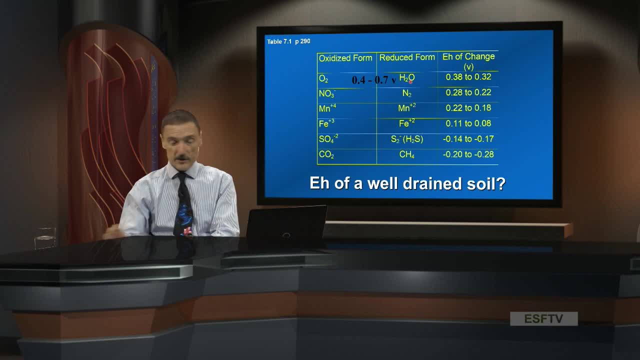 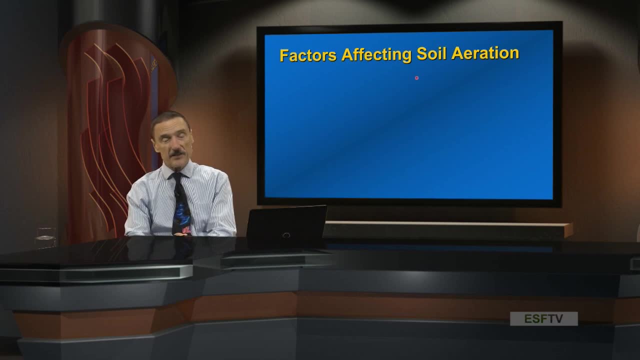 a well-aerated system. So those are very useful points to know. Okay, so we've quantified it, we've kind of described it, we've looked at it from all ways of thinking about the process and now we'd like to wrap that back up. 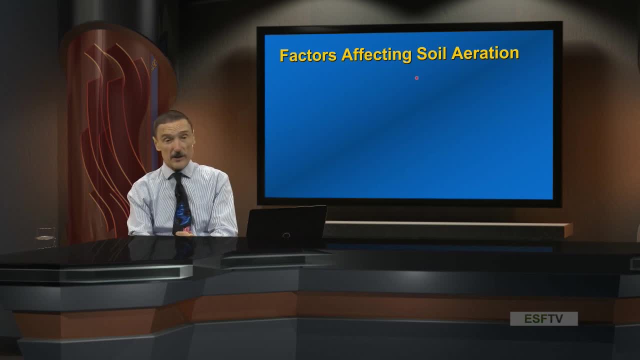 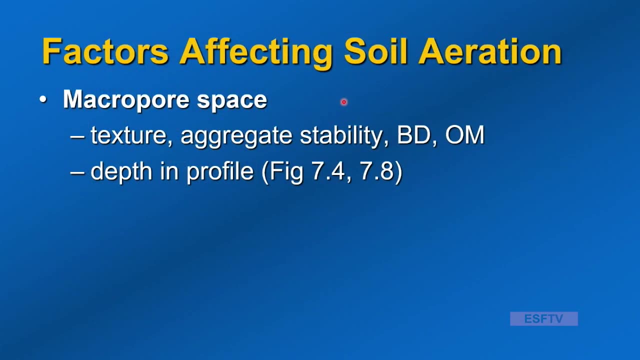 come back to the beginning and think about what are the factors that are important, And so, in reiterating this, we'd have to talk about macropore space, And so what's controlling macropore space And things we've talked about already. 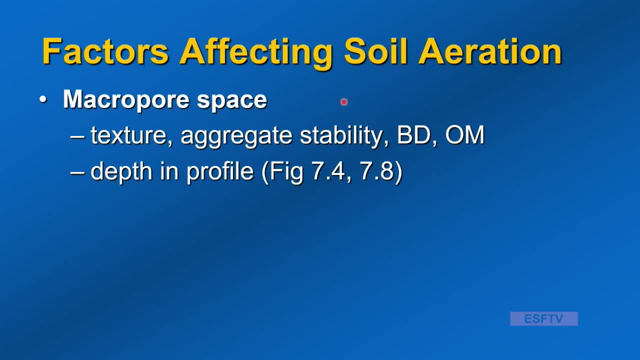 in physical properties and continue to talk about: in soil, water, it's texture, it's aggregate stability and structure, it's bulk density and organic matter. So these are the big drivers from our physical properties: understanding of macropore, space, Texture, sandy soils. 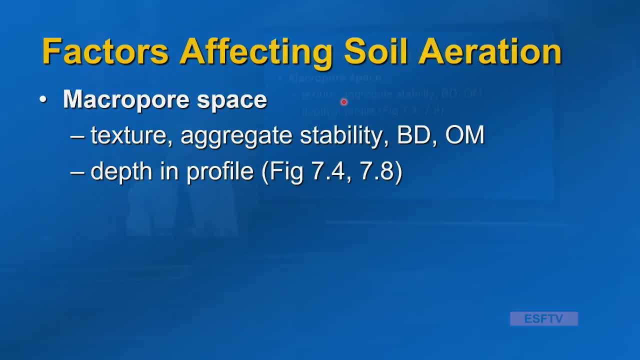 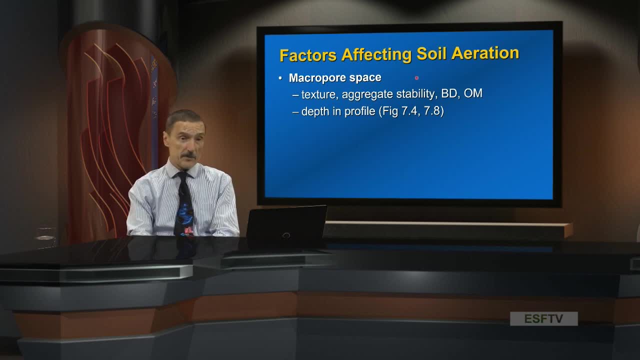 greater proportion of macropores. Stable granular structure and fine textured soils. stable macropore space. Lower bulk densities. generally more total pore space and we try to think about a lot of times more macropore space And organic matter. 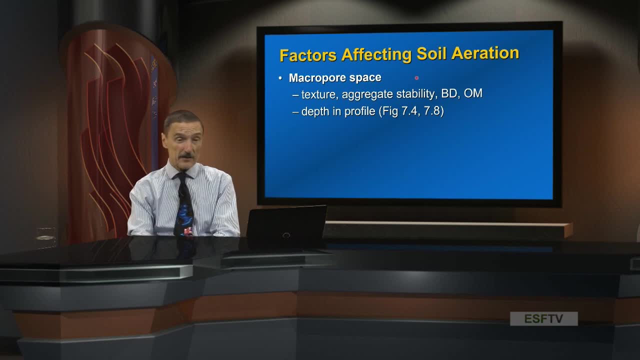 low density contributes to structure and organic matter. So again, we connect these ideas with a well aerated soil, with soil physical properties, And it's important to keep this in mind. We'll come back to this So in the final exam. 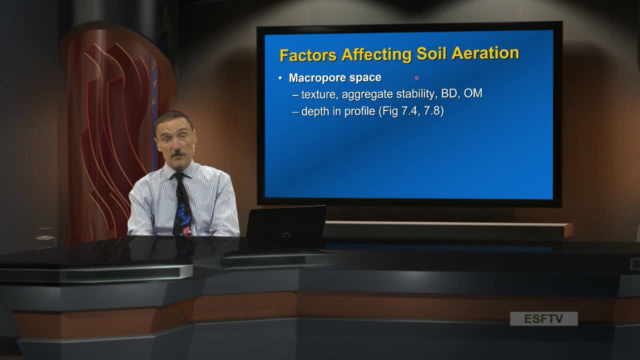 the cumulative final. you'll have to kind of recall some of this and think about the factors that contribute to aeration and relate those to physical properties, And then depth in the profile. That was the last thing we talked about in the CO2 production. 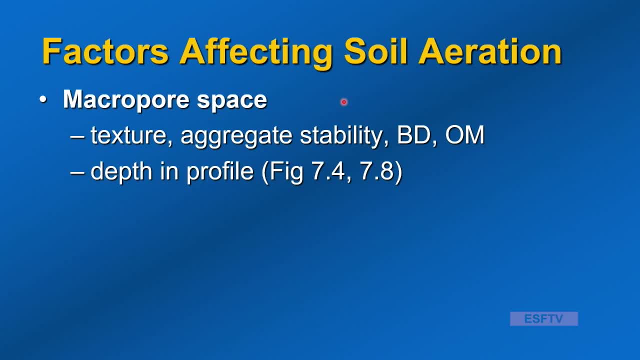 and the last thing we talked about in temperature, And so now we bring it into macropore space and bring that back around. So here we are with the soil physical properties that affect macropore space because they lead directly to well aeration or pore aeration. 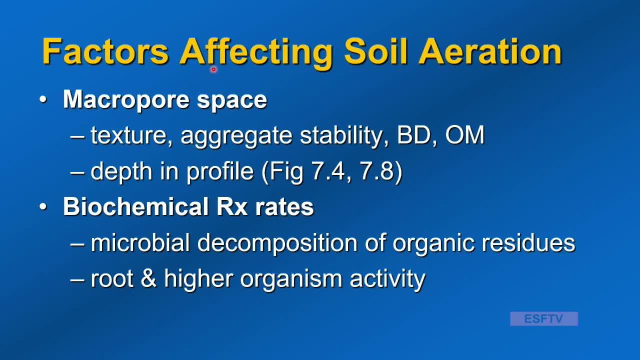 And then the consumers, the biochemical reaction rates. Who are the users? We've got the roots. we've got the higher organisms, the earthworms and the coleoptera. We have the microbes, the fungi. we have the bacteria. 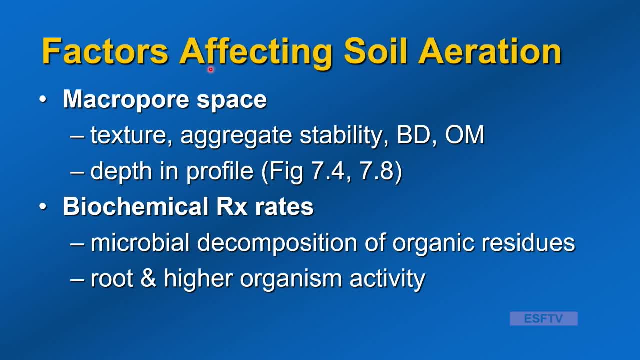 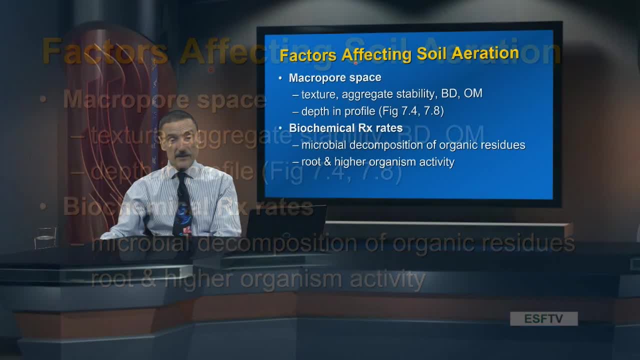 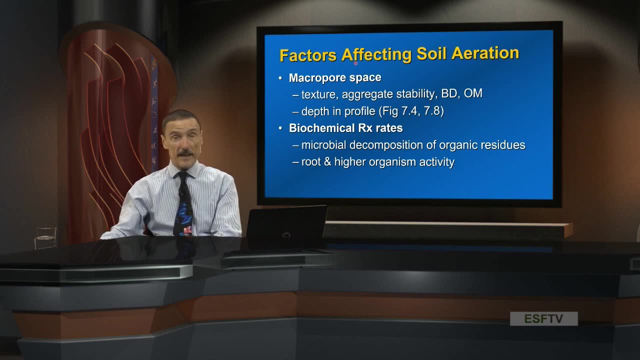 they're decomposing organic residues. All these critters, from micro to macro, are generating carbon dioxide and utilizing oxygen. So the collective intersection of all this is the ability of well aerated soils to continually support high rates of biological activity. So we think about 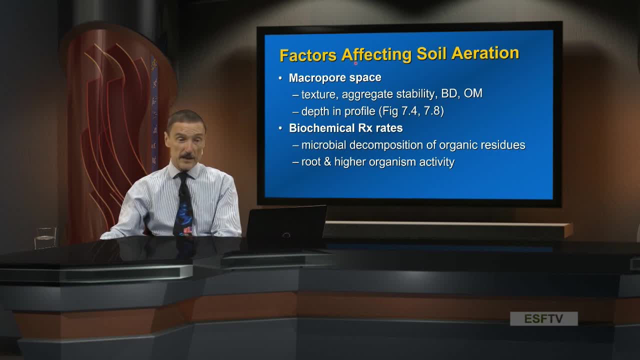 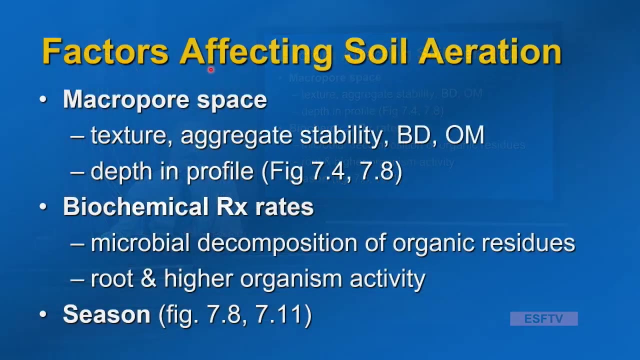 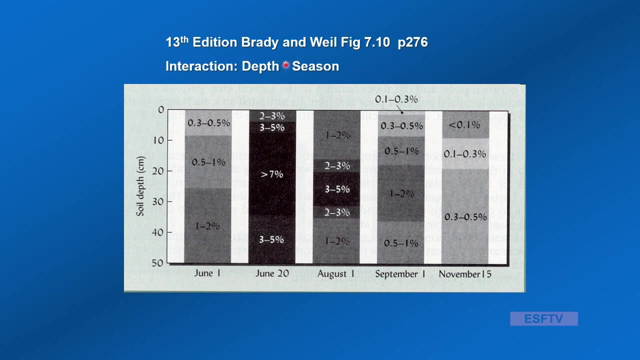 high rates of biological activity. We want to grow food, aerobic systems, well aerated soils, higher rates of productivity And season. These interact with season, not unlike water. Here's a nice illustration. So this is an older one, the 13th edition of Brady.